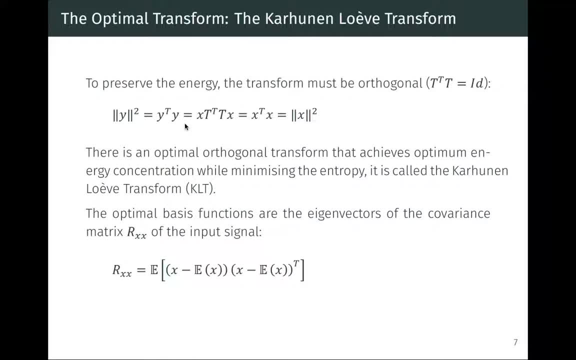 what is the best? best way is the, the Karun-Loeuf transform, which basically looks for trying to do energy compaction, and by energy compaction we means that put most of the variance of your data along one particular axis. okay, So we try to. 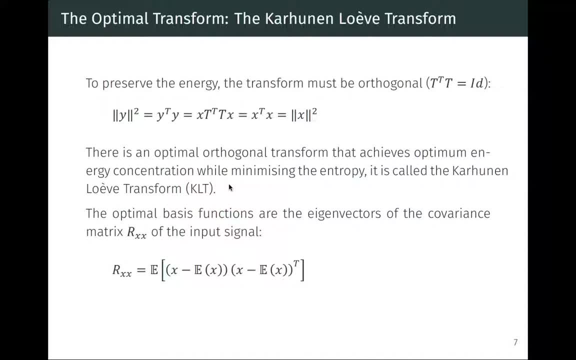 reorganize, to do a transformation of your space into new coordinate system where the axis are ranked from being the most useful or capturing the most variation in the signal to the last one. and last axis represents just the dimension of the noise. okay, so you don't have much going on there. 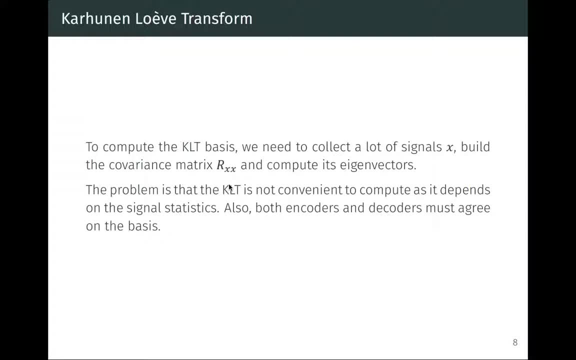 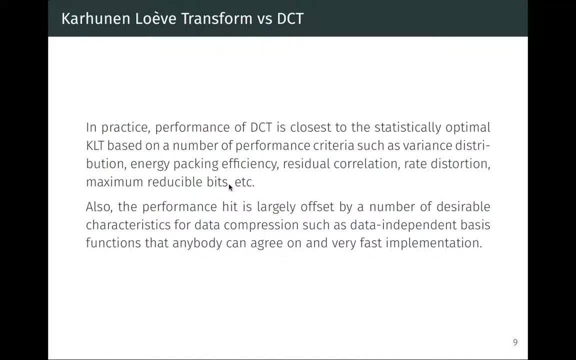 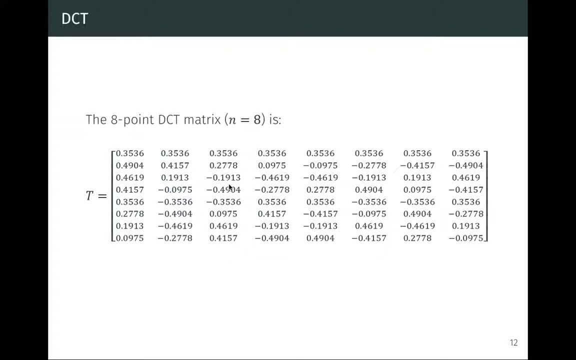 But we said this is kind of hard to get in practice for for coding. so usually what we found is just to use a DCT is just good enough and very close to the optimal and at the benefit of lots of very nice properties in terms of computation and so on. So we looked at that. this is a transformation you have. 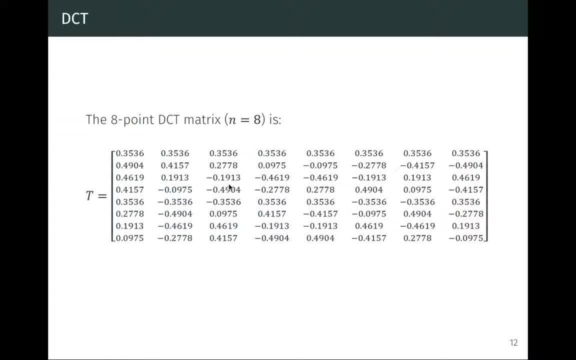 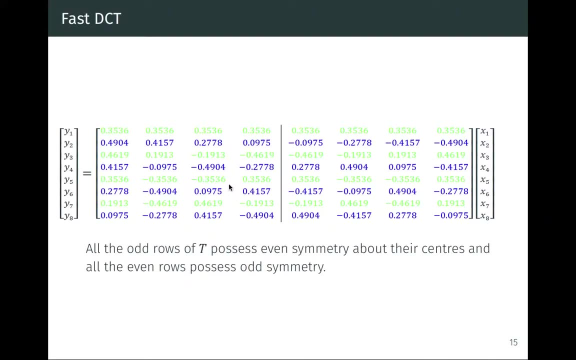 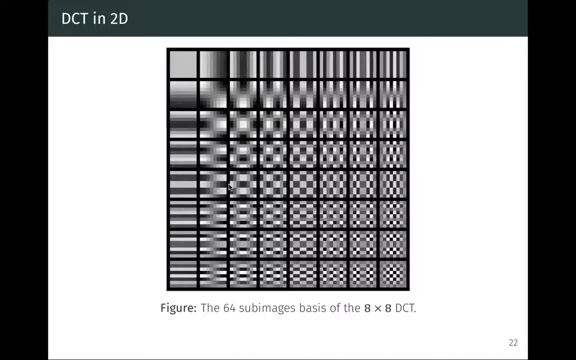 for the eight point matrix. now, remember, this is looking at 1D. when you work at 2D, you have to apply that both in X, in the Y direction, and this is we said: okay, there's some fast ways of going around that. this is what the 2D transform looks. 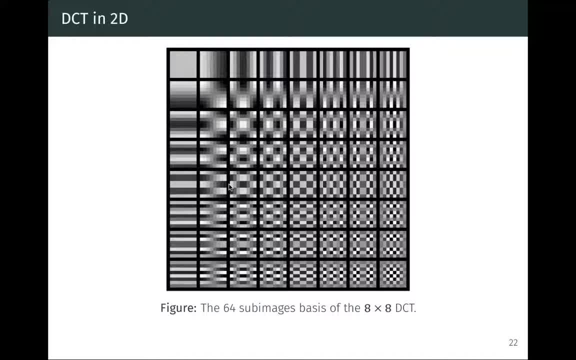 like okay. so basically what I said last Friday, but that if you look at 8 by 8 patch you applying the DCT is equivalent to multiplying the patch by every single of these sub images. okay, and all these sub images you see here, 8 by 8, and the corresponds to the mass, the weights of 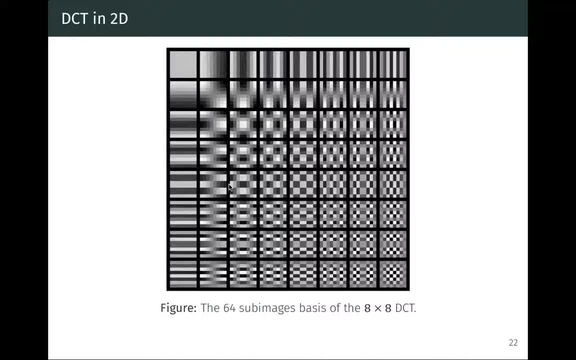 your mask and the weights are basically between. you know the negative or positive. you can see they represent a whole range of different frequencies in your picture. so on the top left you have the low frequency and the bottom right you have the very the highest possible frequencies of your patch. what you say. 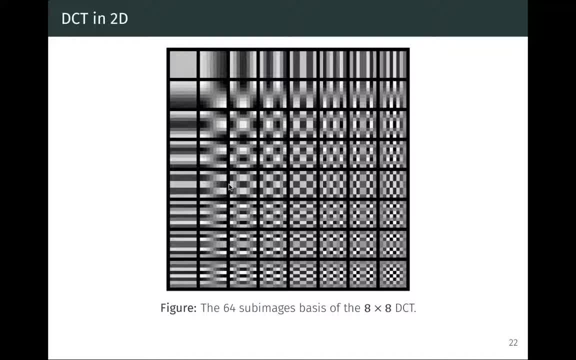 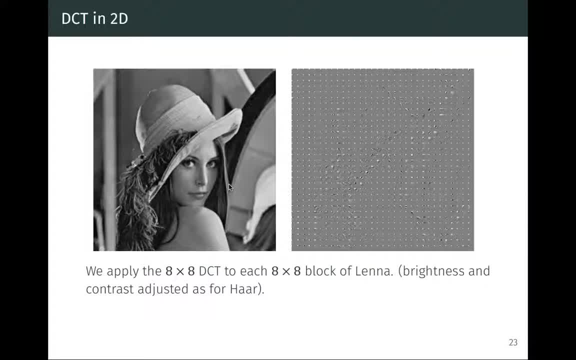 that any patch can be expressed at the linear combination of these little images. okay, so this is what we have. okay, so sorry, I will switch up the the light here. okay, so on the left you have your original picture and on the right what you have is the transform. 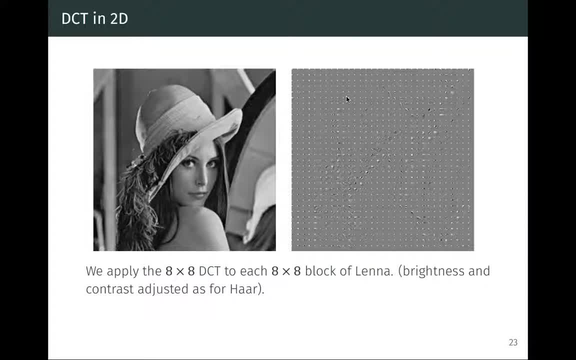 when we replaced in situ all the blocks. okay, so we take we split the picture into 8 by 8 blocks. for each of the blocks, we replace this 8 by 8 block by the transformed by the DCT transform. so when you look in detail at a particular block, 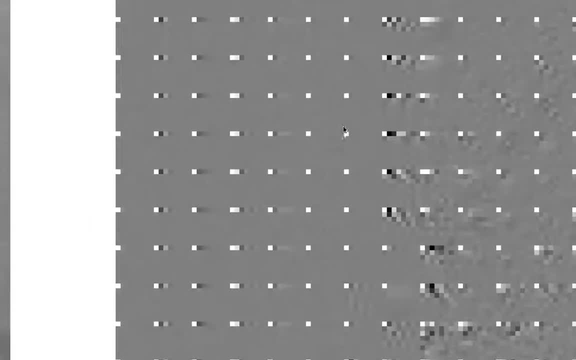 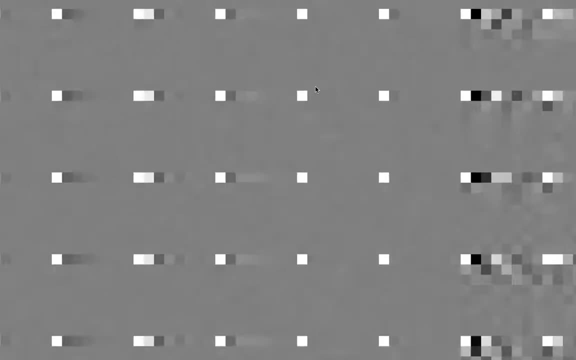 here. what you see the distance here is is 8 pixels. so between the two white points here, this is, is what? eight pixels? and here you have an eight by eight pixel, and the top left corner is: uh, so mid-grave is zero. okay, because you can have negative values and bright means. it's very. 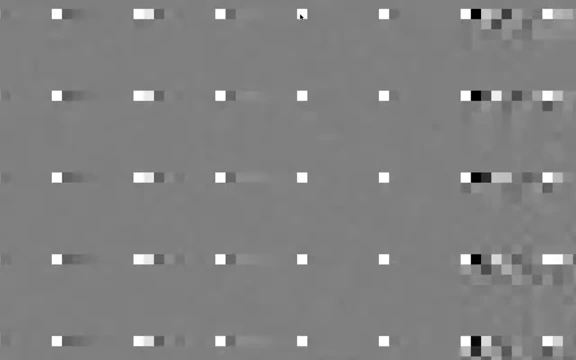 high and you can see, for all the blocks you, you always see one point which is very bright and it means you have one of the coefficients that is very, very important and that's the dc coefficient. okay, so that's the, the low pass of your, the average of your block, and that's. 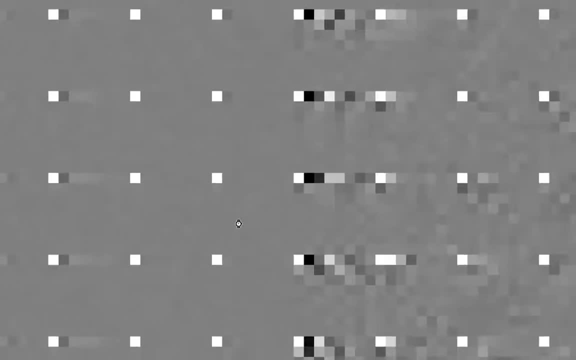 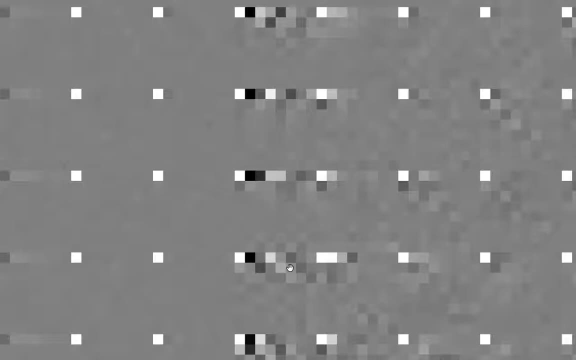 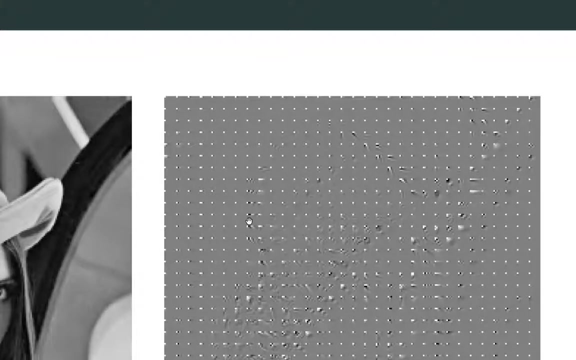 something you can see for most of the blocks, except, of course, when you have, uh, soundflame blocks, where there's a lot of things going on, lots of texture, in which case there's a lot of blocks that have, um, non-zero frequencies. okay, so if you try to see what this block looks like, 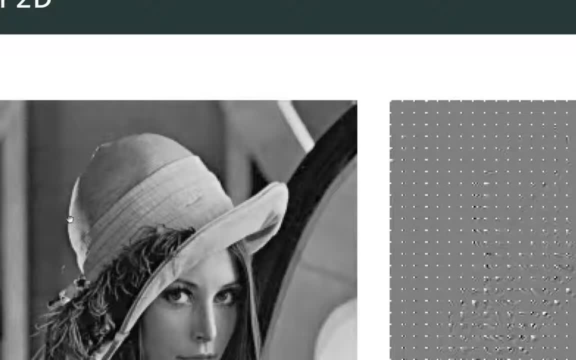 in this image. you see that would correspond to this block here. so, indeed, you see, uh, also you have a, an edge in that picture and therefore, uh, the edge corresponds to a lot of higher, high frequencies, especially in the x-direction. So when you look back at that block, 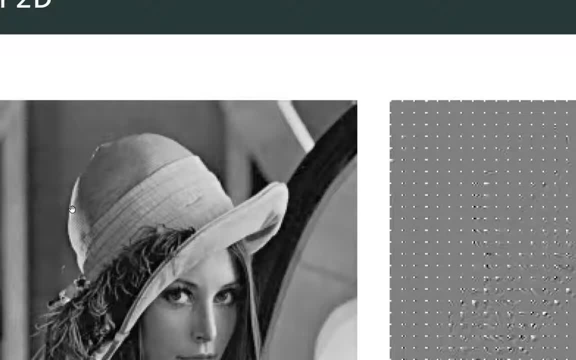 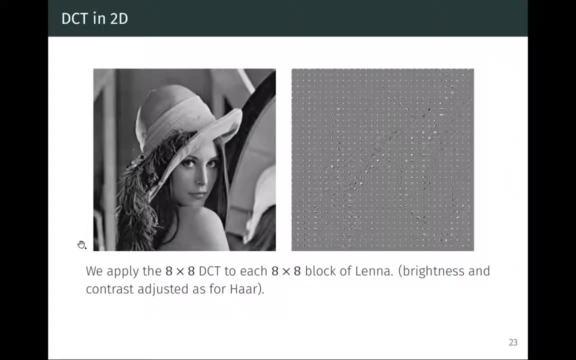 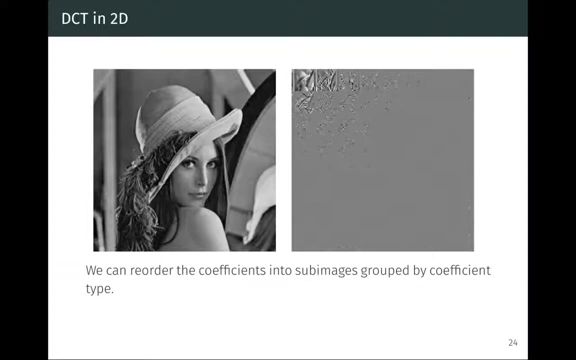 you'll see a lot of the high frequency in x would be quite high, All right. so this is the same image, except we've done the same trick as we've shown with the Haar transform, where we rearrange all the coefficients by type. 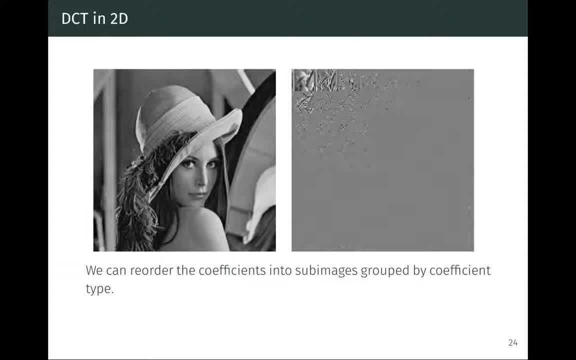 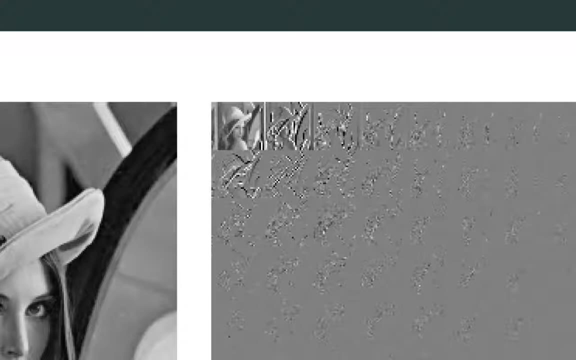 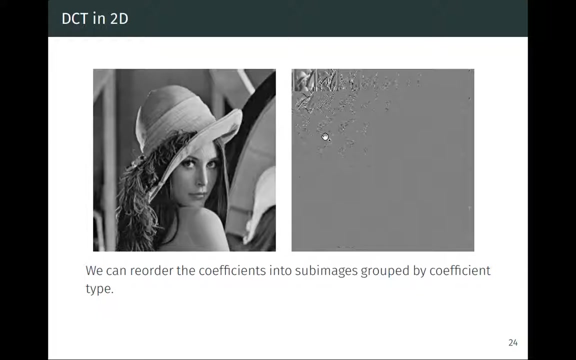 and that means that we took the DC coefficient for all the blocks and we assembled that as a small picture. all right, Now, essentially, what you have here is all right. let me see, Oh sorry, So- what you see here. 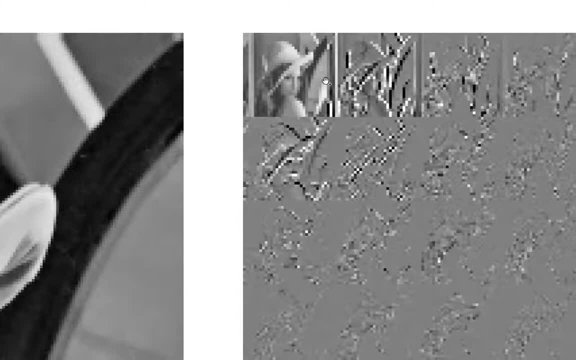 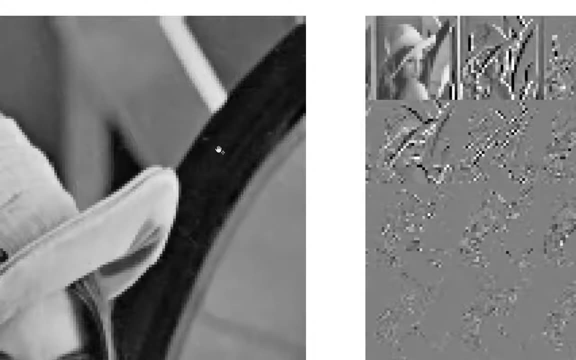 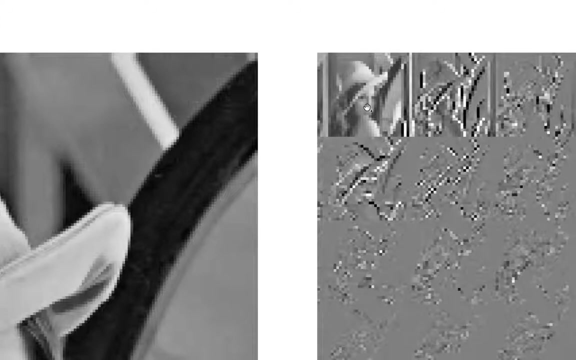 is the picture of all the DC coefficients and therefore this is a picture is eighth of the resolution, in x and y of this original picture. So here we reduced, we divided by eighth the resolution. That's because we take only every single. 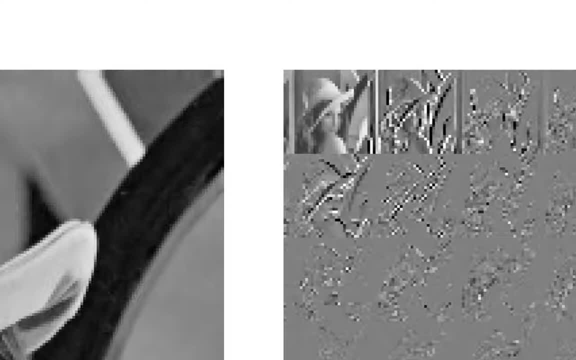 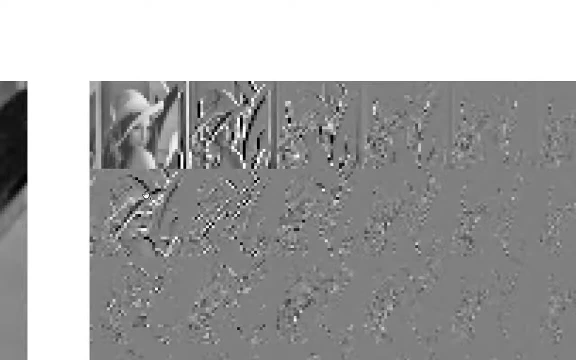 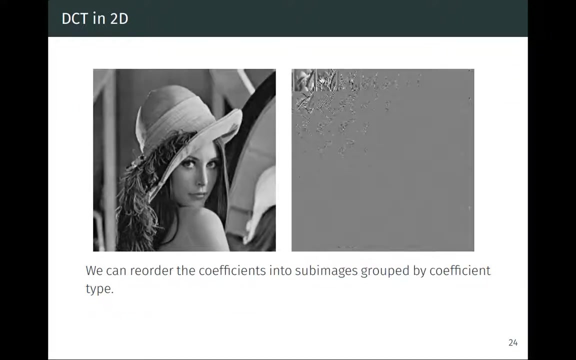 we take blocks of eight by eight And what I say, what is interesting here is that when you look Okay, So basically here you have 8x8 pictures. so when you look back here, you have 8 pictures on the X and 8 on here, so you have 64 set-bound images. 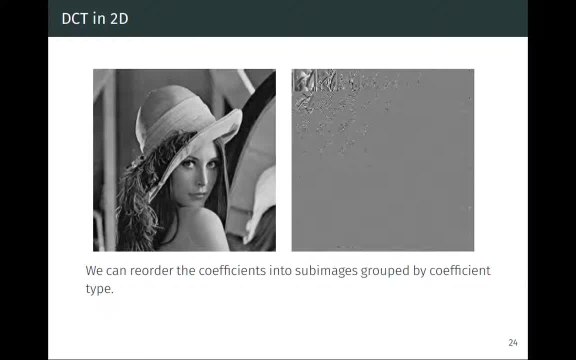 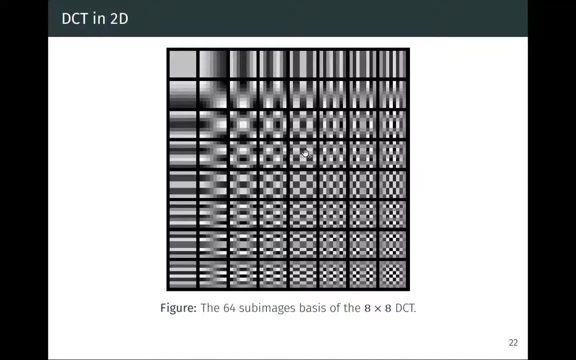 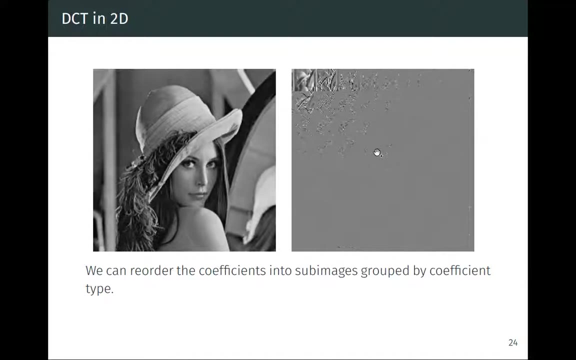 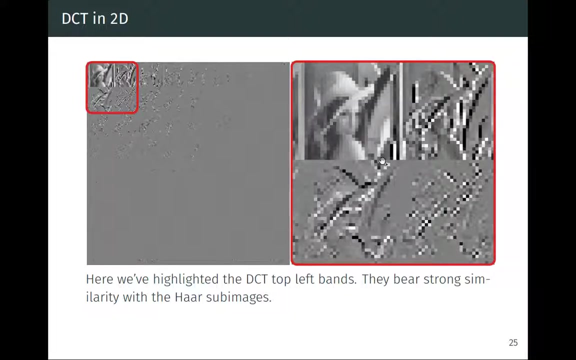 So each of these images corresponds to the response of a particular filter we've defined here. So here you look at a particular frequency and when you look here you get the response for that particular frequency expressed as a semi-version. When you look in detail- and I just isolated the four top left responses- it's very similar. 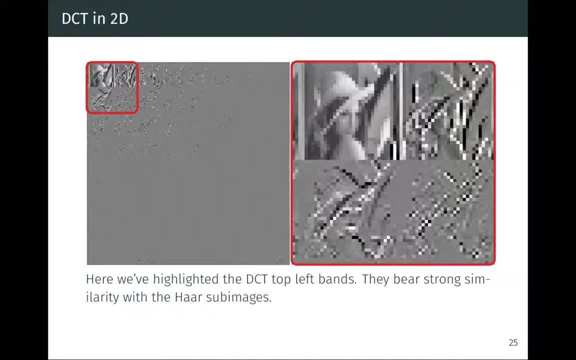 to what you get in Haar. and that makes sense because this more or less does Haar. so it's not quite like Haar, but it almost like Haar. So the top left you have the low, low frequency, so you have a low pass on both X and X. so 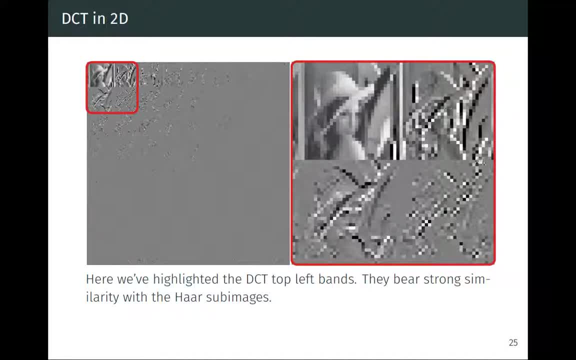 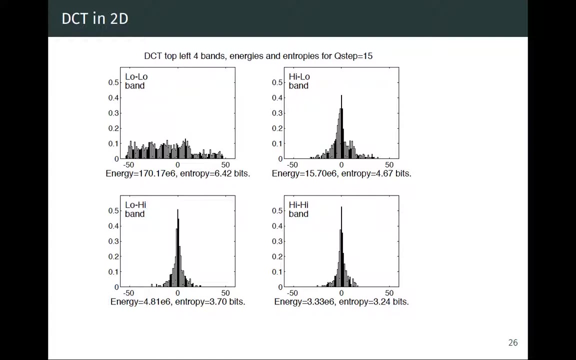 you have X and Y, and here you have the low, high and high, low and high, high, And they're not quite exactly defined as in Haar, but they're very similar in nature. Okay, so let's look at the entropies and the histograms you get for these four particular. 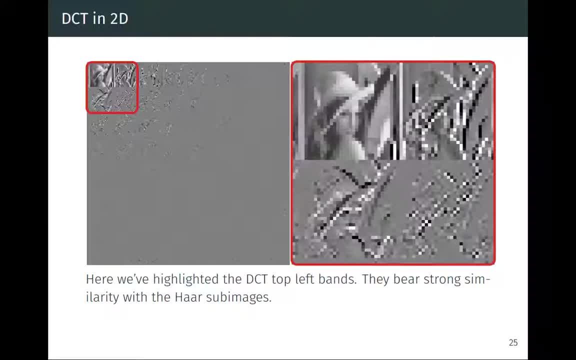 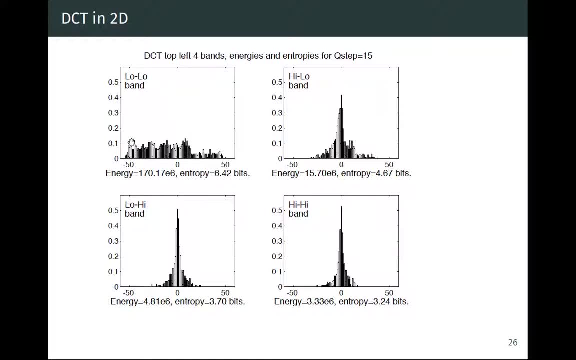 sub-bands. So here we're just looking at the four sub-bands that I highlighted And you see something very similar to Haar. so the histogram for the low low is flat, as the original picture is. and then the histograms for the coefficients for these three particular 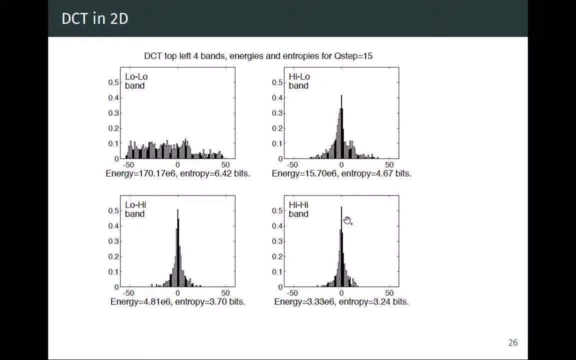 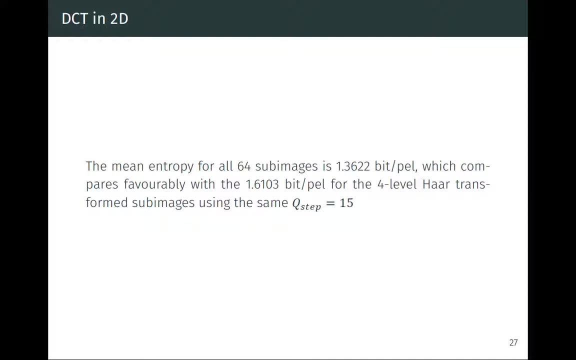 bands you have a peak which is pronounced at zero. so most of the coefficients are near zero and very few are high values. I can see the entropy is quite low In all these other sub-bands. So the average entropy over the 64 sub-bands it's 1.3 bit per pixel, which is a lot better. 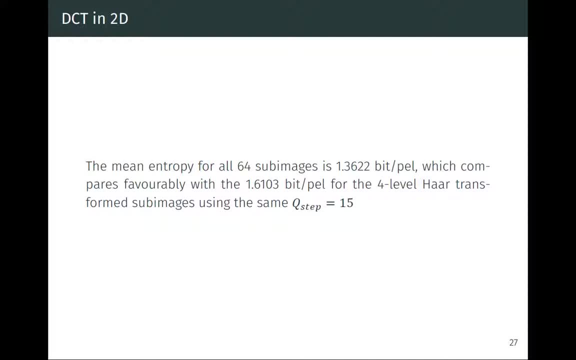 than what we had for Haar, when we had a 1.6 bit per pixel for four level Haar, And that's using the same quantization step. So that's quite good. So we made quite a lot of progress there. But looking at the entropy, we know that the DCT does a fair bit better. 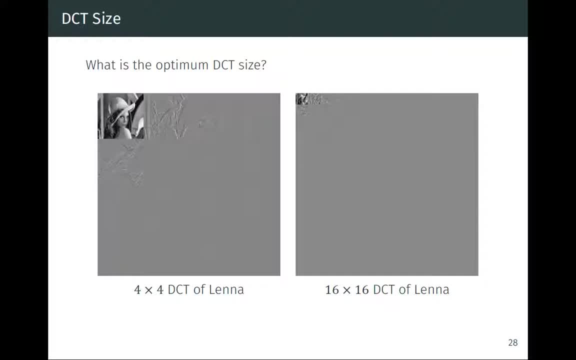 So the way in Haar we had the question of you know how many levels do I do? Now here you don't really do that because already the pictures are quite small. so you don't do a multi-level DCT as such. But in DCT you have one parameter which is interesting, which is the size of your block. 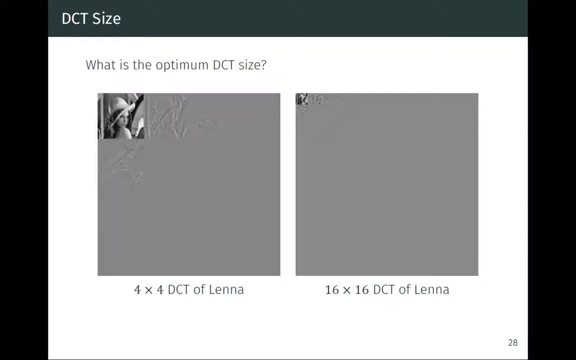 So If you do a A, A two by two DCT, you look at pixels, at, you know, sub-blocks of size two by two. Okay, So you have look at four pixels And that's very much similar to Haar. 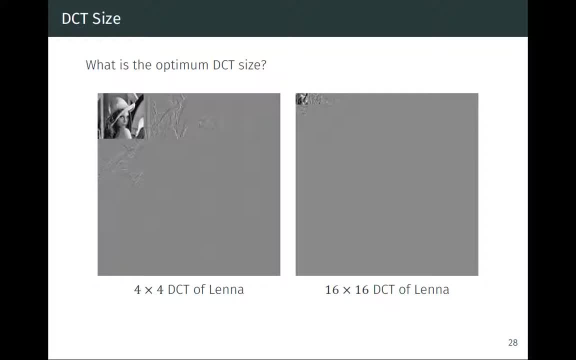 Okay, So we know that we probably want to do better. So you can look here. you have two examples of transform for a four by four DCT. So you're looking at 16 pixels at the time and the 16 by 16.. 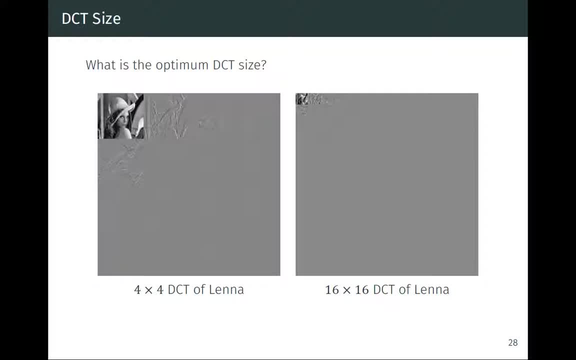 So we look at 128 pixels at a time. Okay So, On the left it's a four by four DCT, So you, the number of sub-images you have, would be 16.. Okay So, four by four, So you have 16 different types of filters you apply and the 16 by 16 DCT, you have 128. 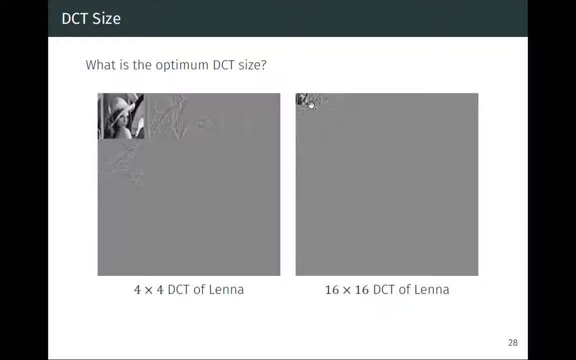 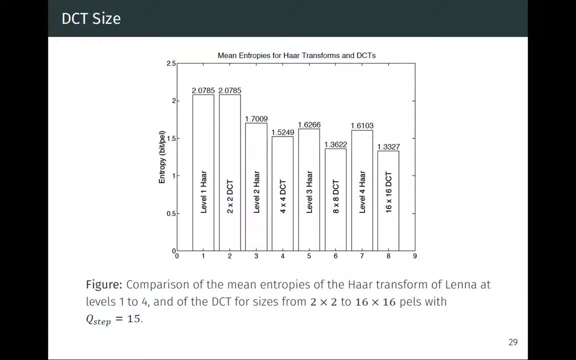 types of pictures, Okay, And each of them being smaller, Right, So? So let's do the numbers. Okay, Let's look at the entropies, because that's kind of the best thing we can do. So on the left, here you have the level one, Haar transform, which is two points. 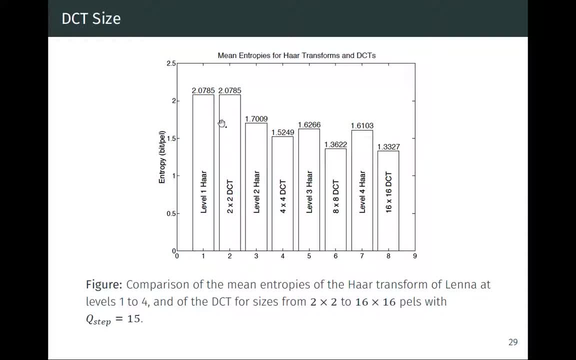 All right, So two bits per pixel, That's for quantization step of 15, sorry. Then you have the two by two DCT, which is roughly the same, And that makes sense. I said the two by two DCT and the level one, Haar, is very much the same in each year. 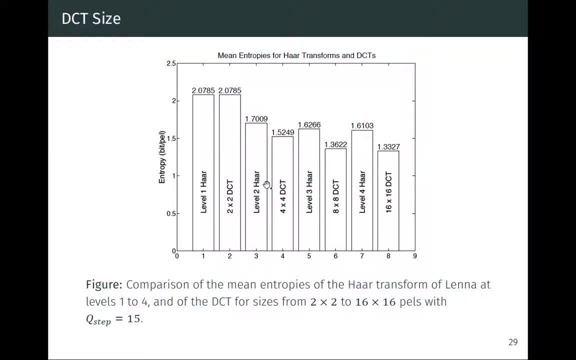 Then you have the level two, Haar, which is a 1.7, the four by four, DCT, which is already quite a lot better than that. Then you climb up to level three of Haar and level eight, And it all seems to go down quite a lot. 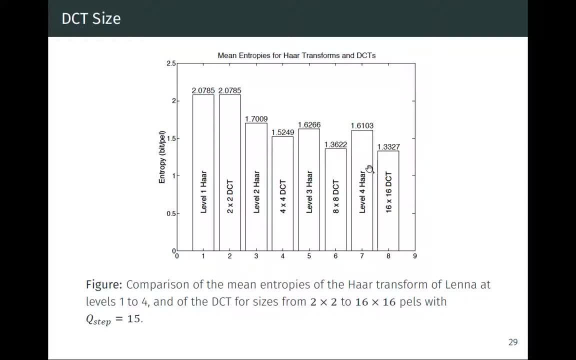 And it's sad to see quite a gap developing between the Haar transform and the DCT. So DCT is quite a fair bit better. So you'd be thinking that, OK, 16 by 16 DCT is slightly better than eight by eight. 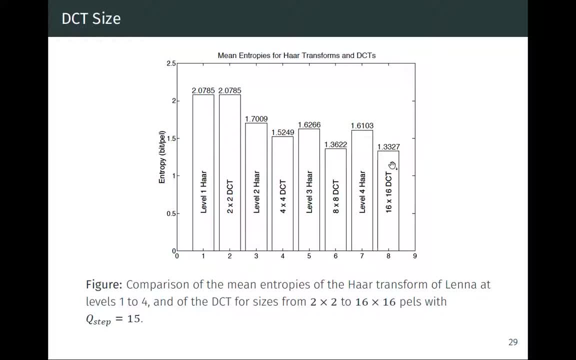 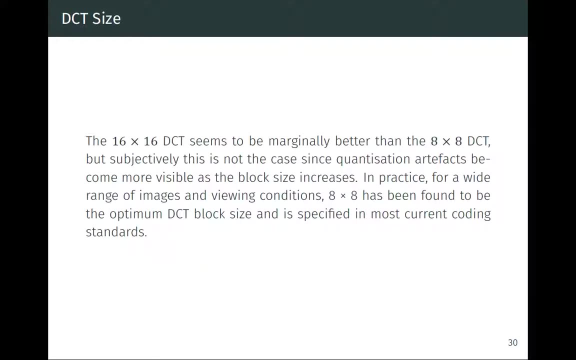 So probably we should take the 16 by 16 DCT. But as it turns out, JPEG uses mostly eight by eight, And the reason why we use eight by eight is because looking at the entropy is one thing, But what we're interested in as well is how humans perceive the errors. 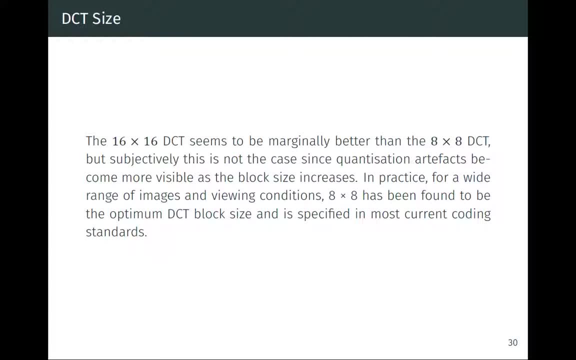 OK, OK. So we're going to look at a number of things And we're going to see what the results of the quantization error into the. you know how to perceive that visually? And, as it turns out, people found that eight by eight DCT error. so the errors: quantization: 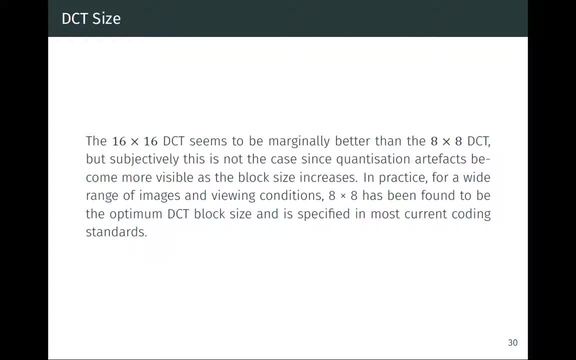 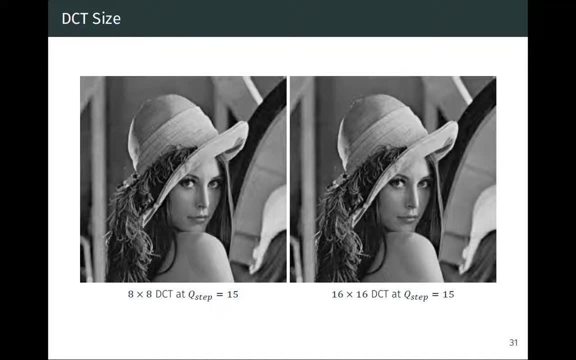 error on the eight by eight blocks are somehow less distracting than the error you get on the 16 by 16.. Try to visualize the very slight differences here. So, as I said before, I use here acrobatics. OK, I use acrobat reader because that's the only one that doesn't the only PDF viewer that. 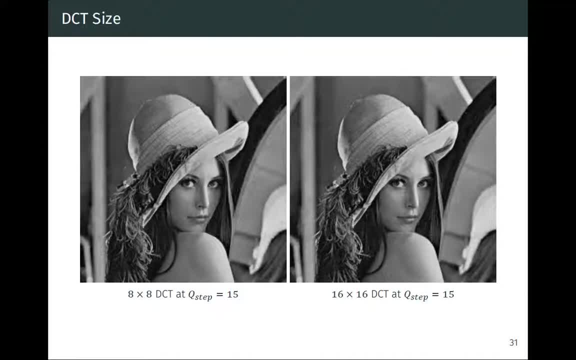 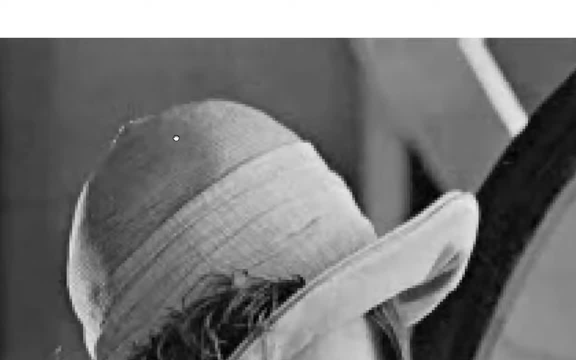 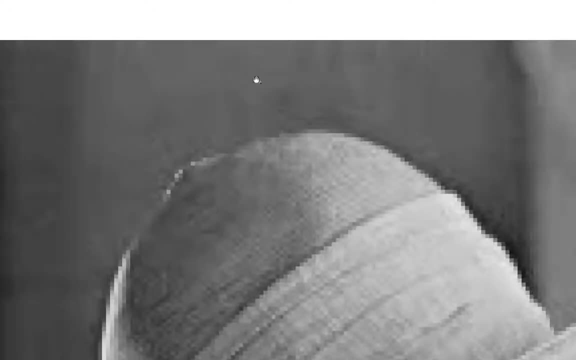 doesn't use some kind of weird interpolation. So you see here the pixels that they are really. So the left here is the eight by eight after quantization. OK, So you can see blocks. OK, So you can see blocking artifacts And. 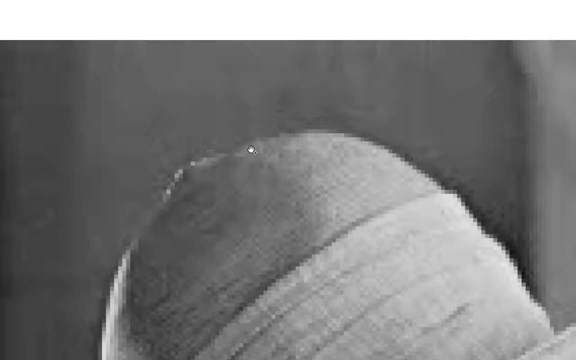 And, And, And. basically, when you have an edge, OK. When you have a smooth area, you will tend to over smooth it at the level of a block, OK. So if you have a very soft, slow gradient going across that, that will result in a lot. 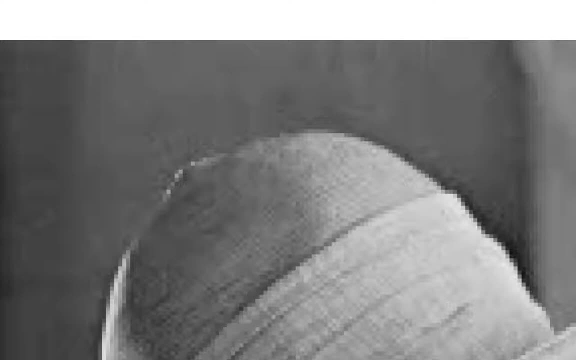 of staircases effects. OK, So you will be trying to smooth too much of that block and you're going to have a staircase effect. If you have a strong edge Because of edge, Because of edge, Because that edge spreads over multiple frequencies, then when you do the reconstruction of it, 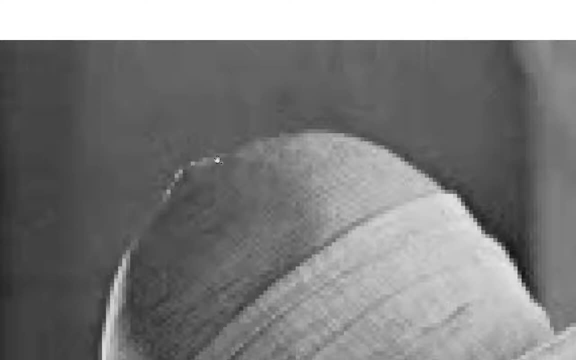 you're going to see a lot of this trickleback pattern. OK, So if you look here, there's a lot of high level frequency that still exists and that's because over the eight by eight block, the frequencies that still show up over the entirety- 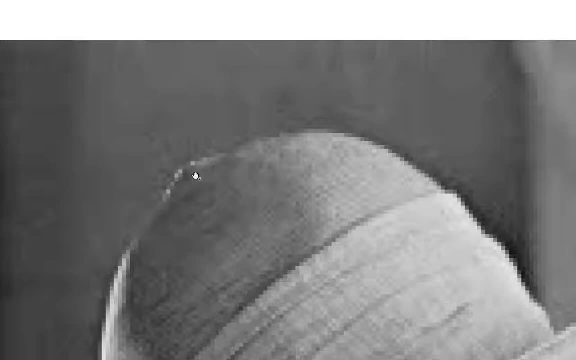 of the block Right. So when you reconstruct that You could see These high frequencies being revealed after quantization and reconstruction, Does it make sense? All right, So all these artifacts are because we don't quantization. OK, If you don't do quantization, obviously you don't have any error. 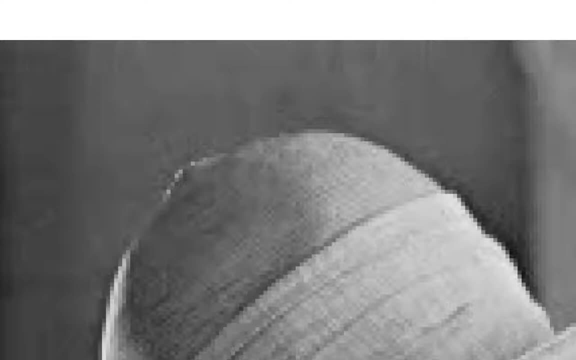 OK, Everything is fine. But here, because we quantize, we're going to cut off some of the frequencies. We can say we don't need those. But obviously when you reconstruct you can see the error. All right. So that's eight by eight. 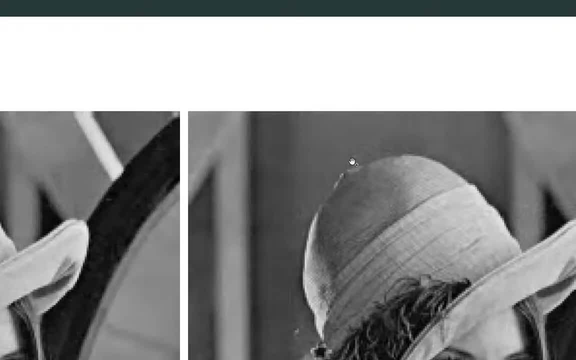 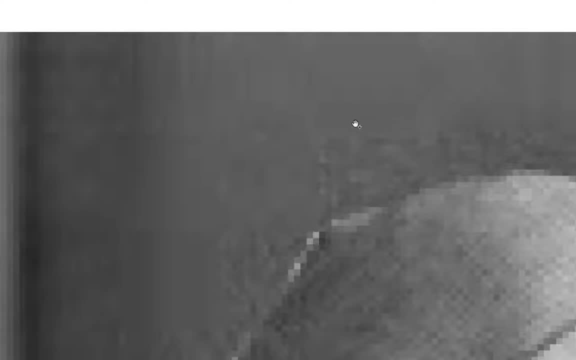 If you look at 16 by 16.. OK, So that's 16 by 16.. OK, So you can see the blocks here are bigger, they're 16 by 16. And that means that the spread of the errors as well is larger. 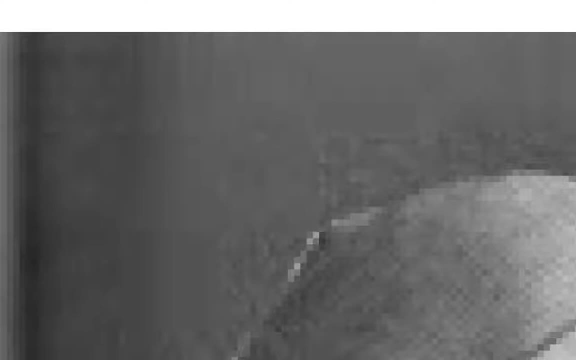 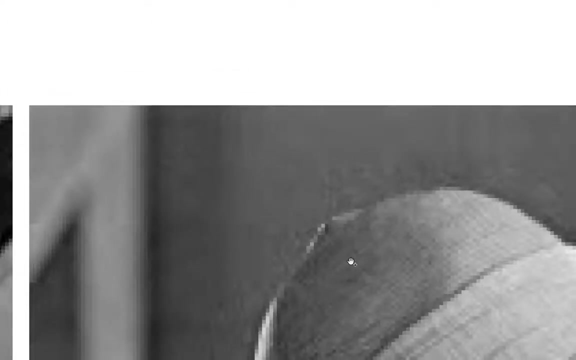 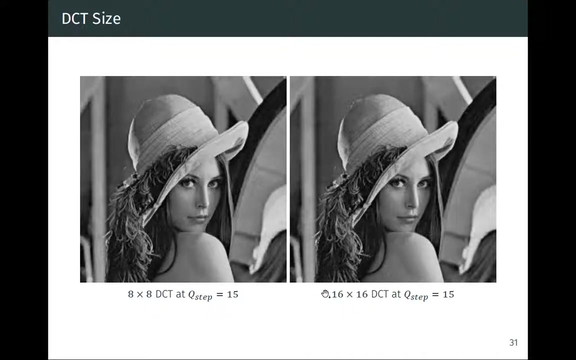 OK, So now you can see kind of ghost frequencies showing up over 16 by 16 block or larger distances. All right, The differences here are very obvious, OK, So differences here are very small. okay, and obviously you know all the tests here. 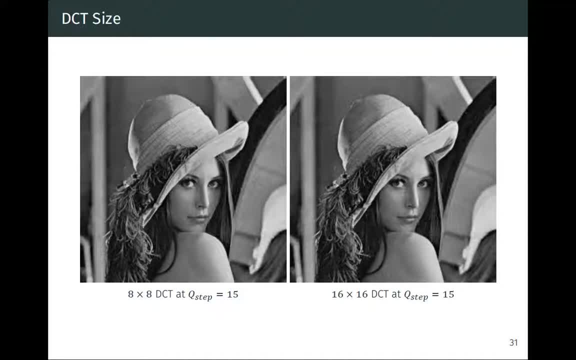 were done by people on calibrated screens and they spend a lot of time, you know, doing all the things I talked about in experiments. so you know, maybe you perceive that as being better for 16 by 16. maybe on a particular picture, is better by 16 by 16. the reason why we went to 8 by 8 is because you know. 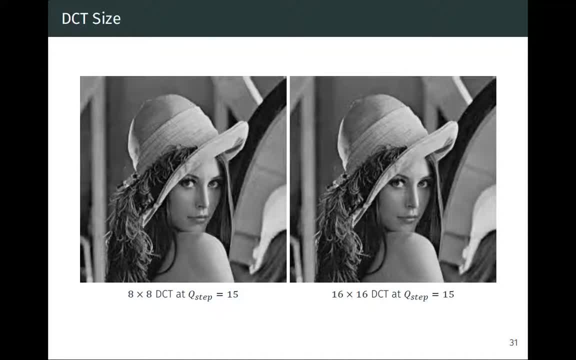 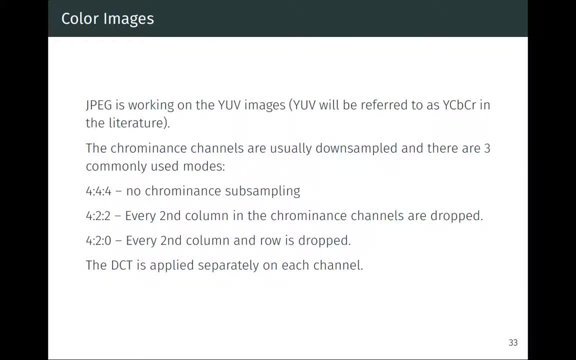 enough people said: okay, it's marginally better on 8 by 8. therefore, okay, we just pick 8 by 8. so these extra more examples of that, all right. so how does it work? on color? okay, so you know, we have principles, so we transform your. 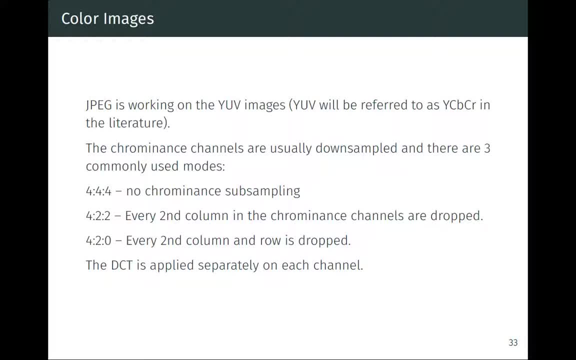 picture in dCT who quantize and come back, and that's fine, that's grayscale, obviously, and real-life. people have color images since quite some amount of time and so, as usual, color we don't do too much. okay, there's nothing crazy going on, because we don't know what's going on with the image in this picture. 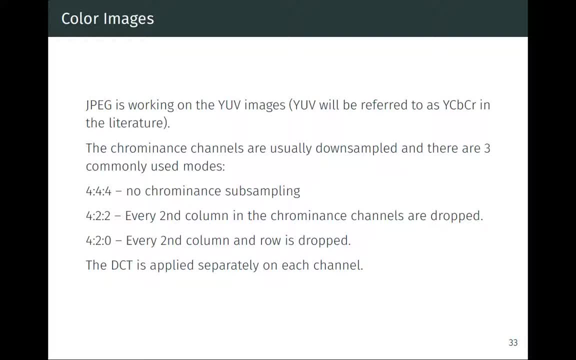 going on. for color, the, the luminance channel, is always the most important one. so what we do here is we, we do the two tricks we've seen. okay, so the first thing is to convert to YUV, so one of the many YUV color spaces. so there's. 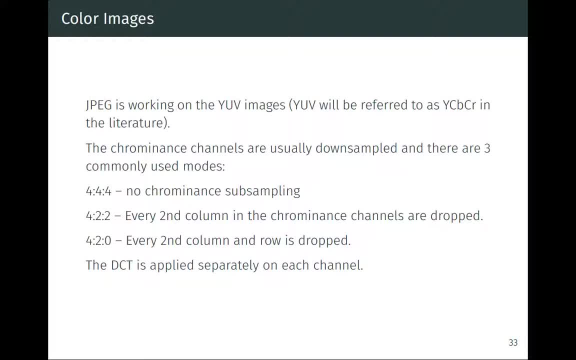 different versions of YUV, as I don't know if you remember the course in that, but one is the YCbCr and that's the one we actually use here for JPEG. okay, so now you have color transformation. you work on the Y channel as you should, and 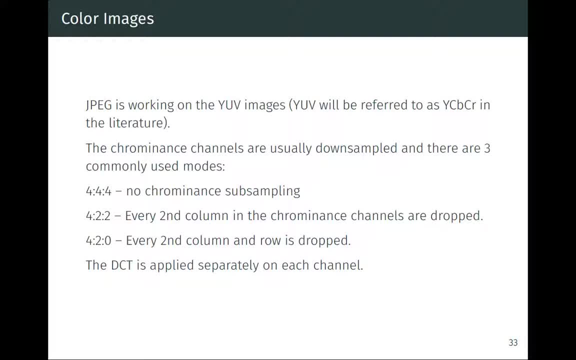 then you can just subsample the chrominance channel, okay, so remember the schemes 4 4 4, 4 2 0, 4 2 2 and so on. okay, basically, when you look at the 4 2 0, 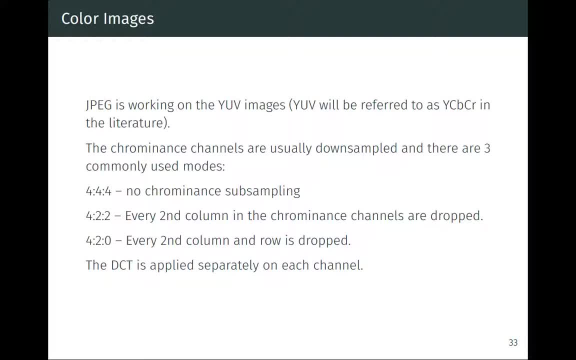 which would be the most frequent one. you subsample by, effectively by two in each direction, the, the U and V channels. okay, so you have your U and V channels. okay, so you have your U and V channels. okay, so you have your two color channels, so U and V, and you're going to take half the resolution both. 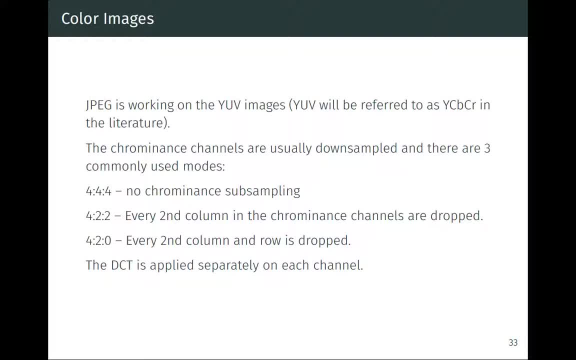 in X and Y. okay, so you can subsample that and now you have three pictures. you have the luminance picture where you can apply your DCT, and then you have two smaller pictures where you can apply the DCT as well. okay, so this is how you do. 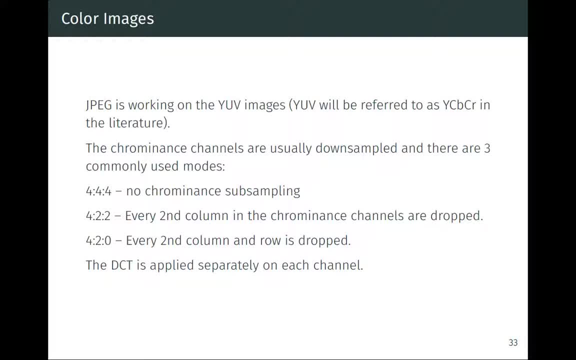 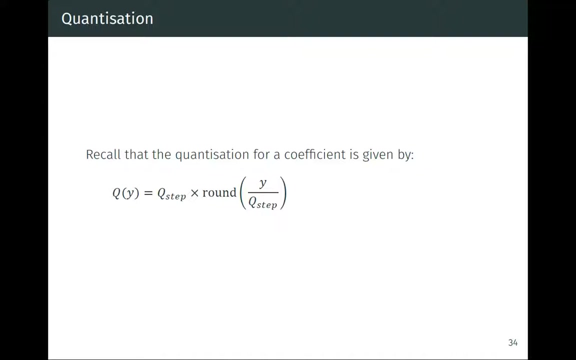 things. does it make sense? okay, so again here, this is where JPEG is really making full use of all the the knowledge we have on how we perceive, how humans perceive pictures and so on. okay, here's all about perception and not about the exact reconstruction, so let's look at a bit deeper into that, okay, so 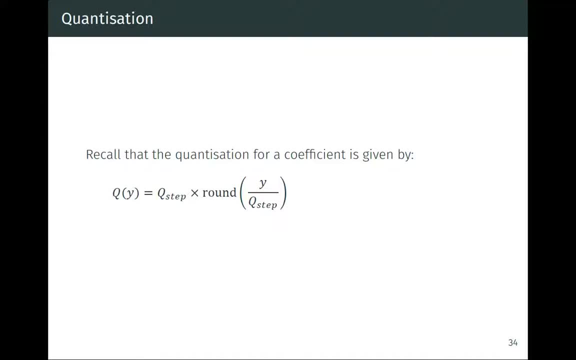 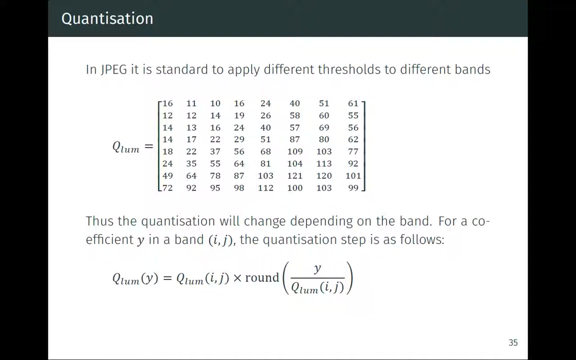 remember the quantization of the coefficients, okay, so the the formula is here. we just, you know, round division and multiply again, and then you have the, the. you might want to apply different thresholds at different bands, okay. so the idea here now is, like you can, to have you have different frequencies both. 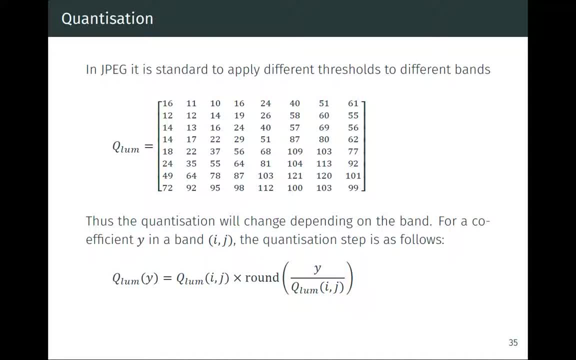 in X and Y directions and you might want to apply, instead of applying the same quantization for all the bands, you might want to do, you know, to be a bit more aggressive at some frequencies and remember that makes sense because we know that we're not as sensitive to very high. 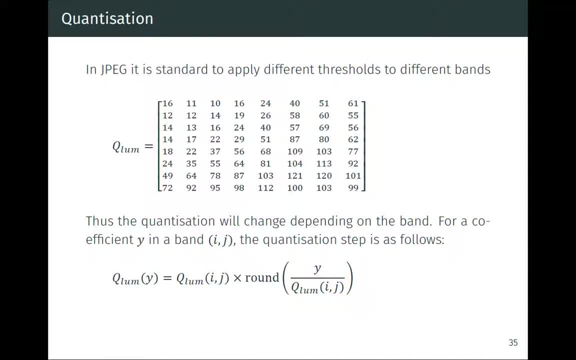 frequencies, for instance, that we are through some low frequencies. so maybe we can gain by being more aggressive on the quantization on these higher frequencies that we are on the low. so what you see here, it's the, it's called Qlum and it's the quantization step you have for the luminance channel pair bands. okay, so 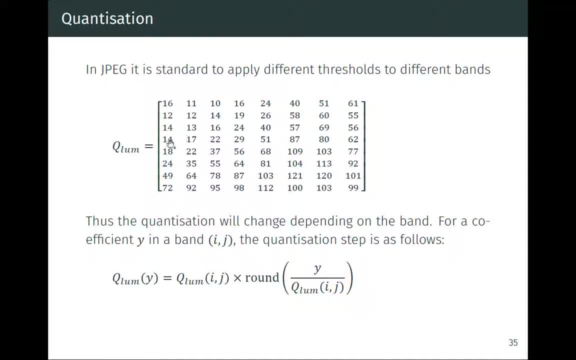 it's looking at an 8 by 8 DCT transform and so here we have an 8 by 8 matrix and in this case, as we said, we need to set bigger time, also when we are putting and we start to apply some testing values in this paradigm. 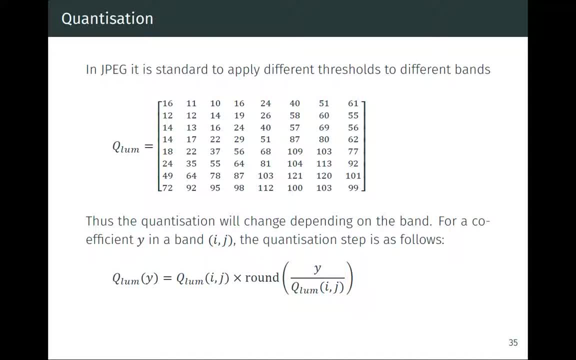 so this is a Q step where we put here all the the Q step for each of the bands. so you remember, this is a Q step, so you divide the number by the Q step and do it again. so this is the Q step you use for a particular band. so what does it mean? okay, so it means. when you look at 16 here at the top, it means that when you look at род GO THESE. 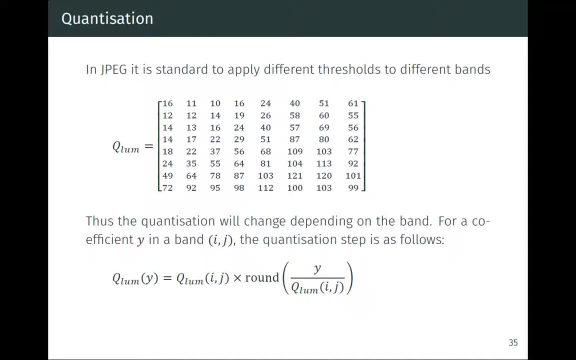 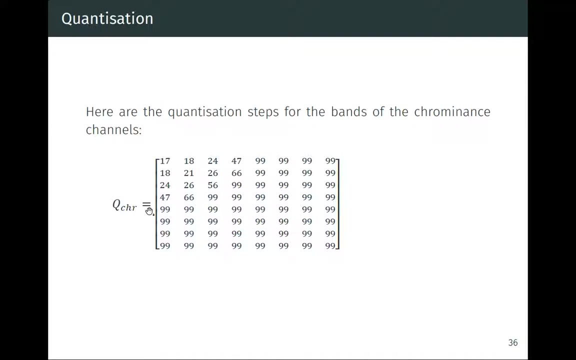 London. the bigger the number, the bigger the quantization is. and in this matrix here we're looking at integer values, right? so the bigger the number, the more aggressive you are. so when you look at the color ones, okay, the color one seems a bit more simple. okay, so you have the same value, 99, everywhere, okay. 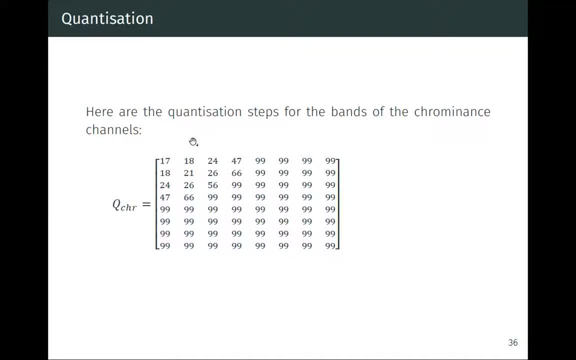 except for, except for the beginning, for the, and the beginning, here is the, the lowest, this is a gc coefficient. okay, this is the kind of the, the, the mid frequencies and this is the high frequencies you have here, okay, so here you're very quickly, uh, are very aggressive for any high frequencies. 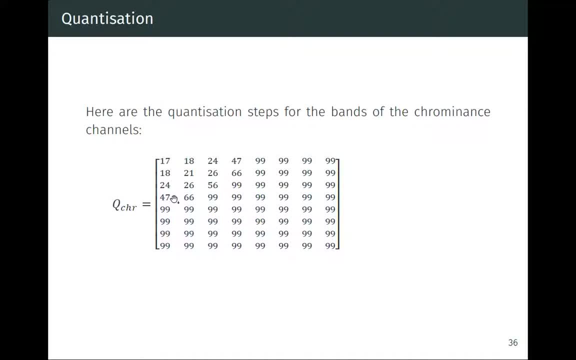 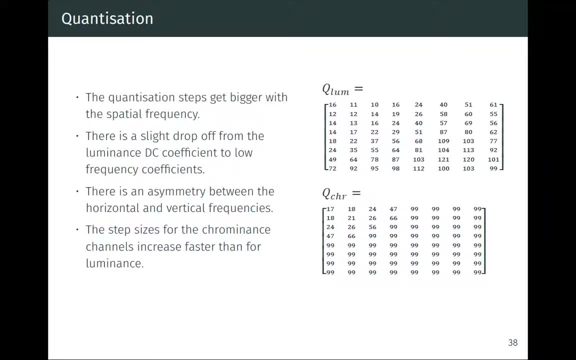 in the color, but you're trying to preserve a tiny bit of the low frequency so just want to you to look at. so i just put them side by side here, just make a few notes here and uh, it really comes back to, um, what we've seen before. okay, so the first remark here is like the 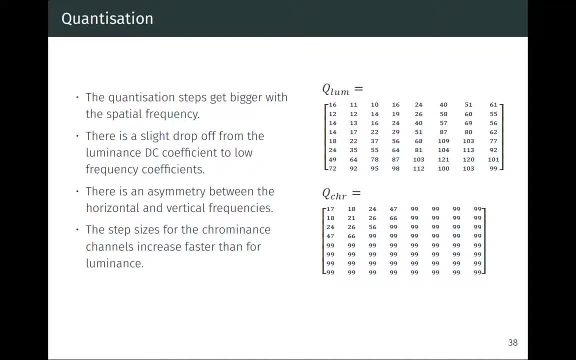 quantization. so it says here on the left: okay, so the, the quantization steps get bigger with the frequency, and indeed in both case roughly, when you go along that direction. just look at the x and axis, you quantize a bit. you know you get more and more aggressive as you, as you get to higher. 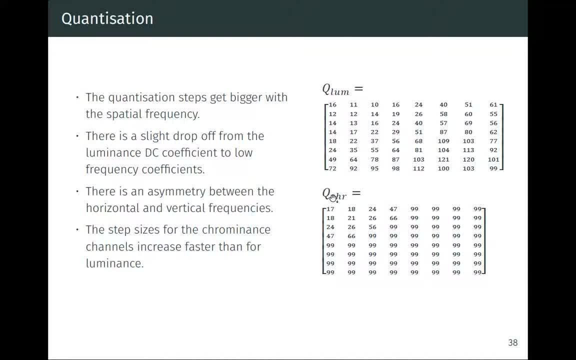 frequencies: okay, and same for the both limits in the in the components. second point: here it's like when you look at the luminance there's a slight drop. okay, so the this value is 16 and then the next one up is 11, 10. so actually there's a drop, okay, so actually you somehow, uh, it corresponds. 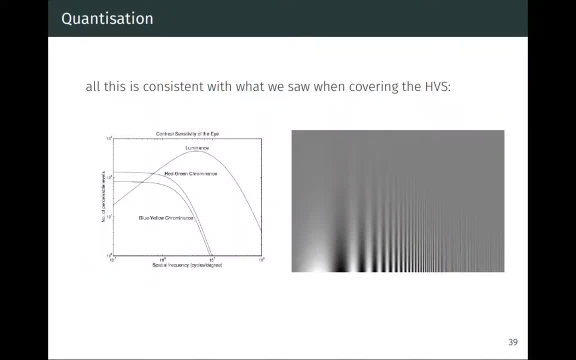 to what we know of the human visual Coordinates to the human visual with the station human visual perception system. so I mean, remember these graphs. you are more sensitive somehow in the luminance to this part of the graph, so you're more kind of sensitive to. 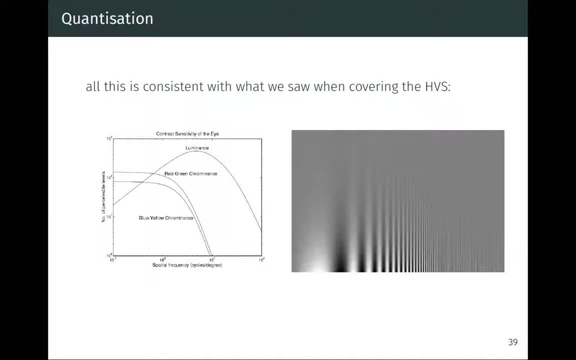 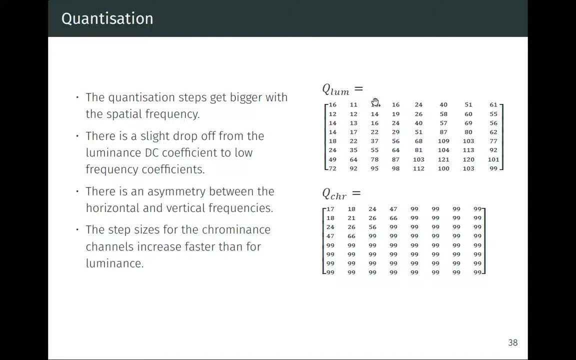 the low to mid range frequencies. So this is the same. here you have this: drop lower values, which means that you're trying to protect these frequencies a bit more, and then you'll be a bit more aggressive. Interestingly as well, there is some asymmetry for the luminance between the x and the y. 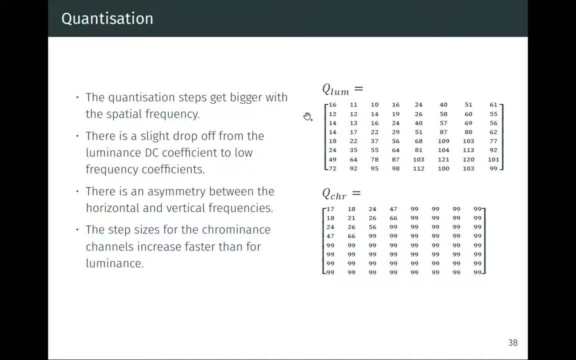 axis. so it turns out the human eye is a bit more sensitive to the horizontal frequencies than you are to the vertical frequencies. it's a bit weird, but yeah. So it's significant enough that it shows up in these coefficients so you can see here. 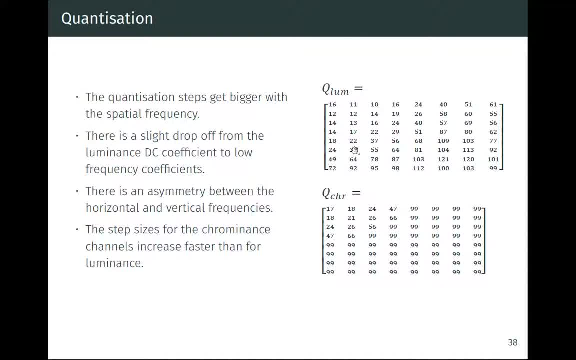 for instance, the higher frequencies, the lower frequencies, the higher frequencies, higher frequency. quantization 72 for the y axis and 61 for the horizontal axis. so you quantize a bit heavier the y axis than to the x axis. And obviously the last point is where you're way more aggressive for colour than you are. 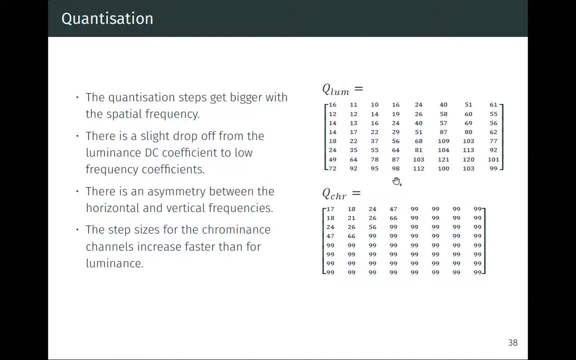 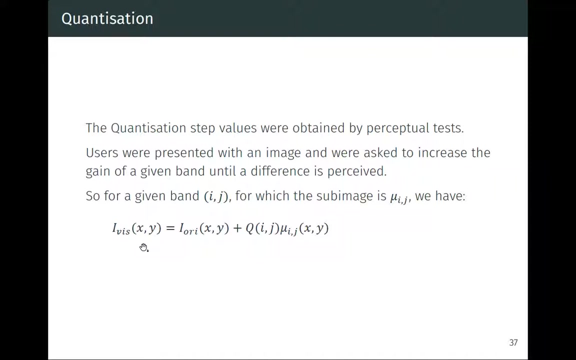 for luminance. So all that comes back to what we've seen from actual pressure choice studies. So how did we get these numbers? Well, We didn't just derive these numbers from that from here, so we actually had a simple experiment. So what they looked at is: you take an original picture and you add, so you look at a quantization. 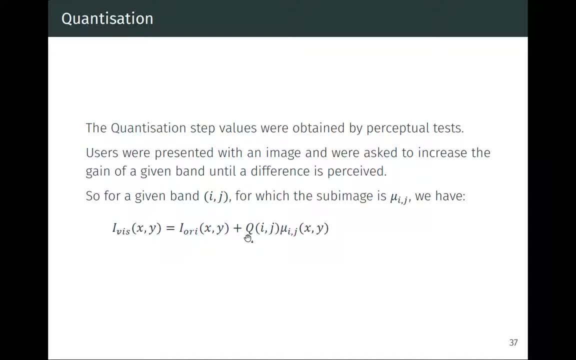 step for that particular pixel or band. so you're looking at a particular frequency band, so let's call it ij. So ij is for the frequency in x and y, And so, for instance, 00 would be your DC coefficient. So that is just to identify the band of the we're looking at. 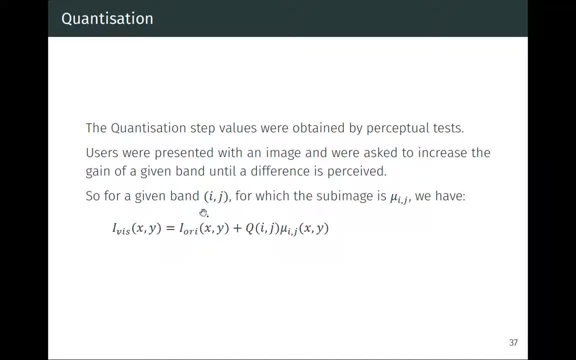 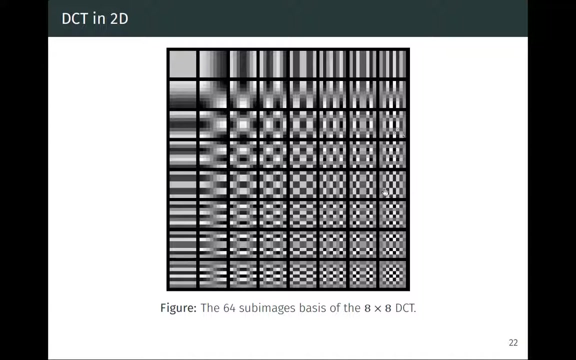 And then we're going to look at the mask, a image or the weight, sorry for that particular band. So, coming back here, Basically we take, you know, we split the picture into eight by eight. So that's where we are. 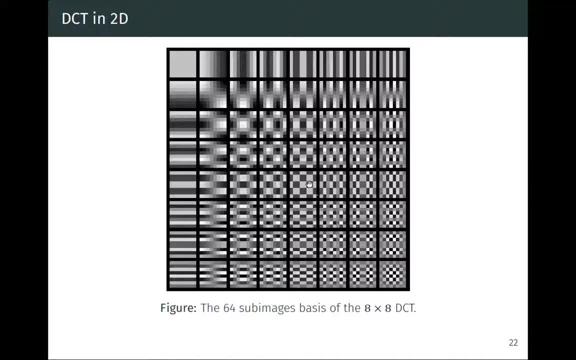 So basically, here's what you look at. So here's what you've got: eight blocks and we can take one of the blocks of you know, one of the bands of consideration, so say this band here, and we're going to add that to every single. 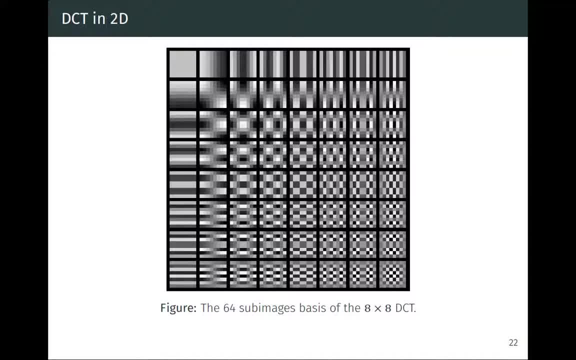 block and we're just going to add that a tiny bit. so we're going to have a weighting factor, global factor, like an amount. we say we add 0.2 of that weight to every single of my blocks. all right, so say that again. we try to assess the. 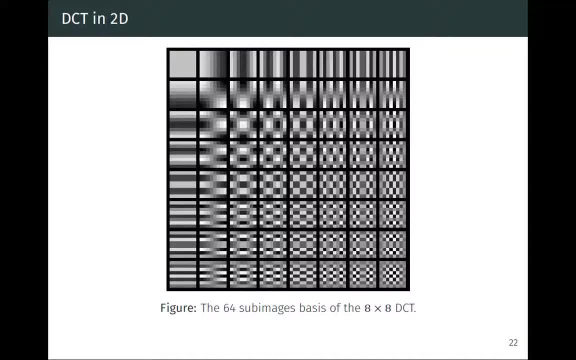 visibility of each band, okay, and to see how we perceive these frequencies. so what we do is we take the original picture, say the linear picture, and we're going to split that picture into eight by eight blocks and for each of the eight by eight blocks we're going to add some amounts of that of a. 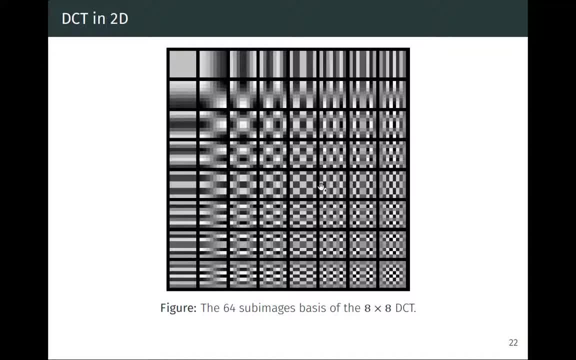 particular frequency. okay, so we're going to degrade the picture with that particular amount. okay, in a linear way, and we can increase the amount we add. okay, so we could multiply that weights by some factor and when the, the user, or the, the, the human, says: okay, I can see a difference. so we'll see side by side the two. 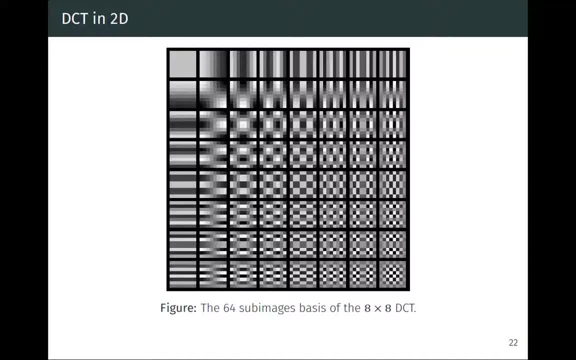 pictures, the one with no alteration, the other one with the same picture where we added that frequency- and then we see, okay, can you see difference? and then at some point you say, okay, yeah, I can see, this one has an artifact and this one is doesn't have an artifact. okay, and we just note when, take note of when, when, 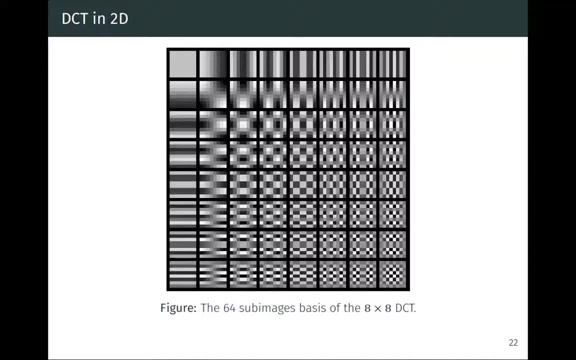 the people can can see the difference. does it make sense what I'm saying here? it's been the same experiment as people trying to recover from the RGB. you know the, the matching functions. okay, here you have two versions. you have the clean version and the version where you add a particular frequency or particular band. 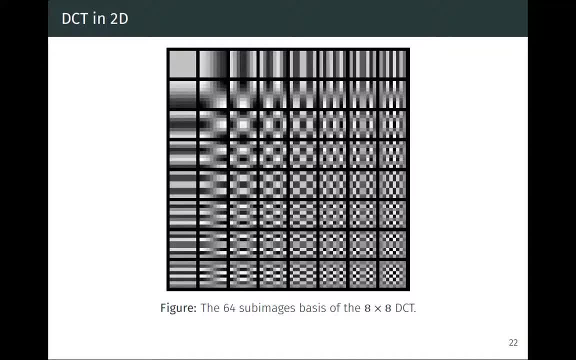 okay to that image, just add it okay, and then we see if we add ten times that version, then we start to see a defect. and if we just add a small amount, we don't see the defect and we just note when people can make a difference. so 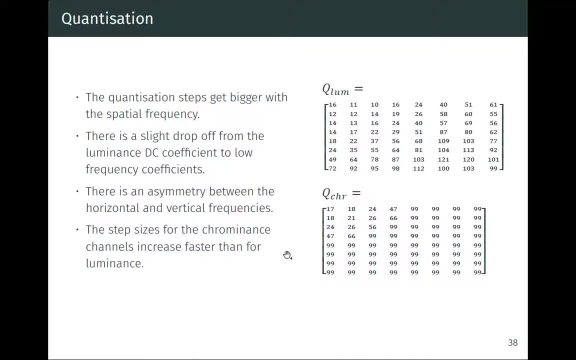 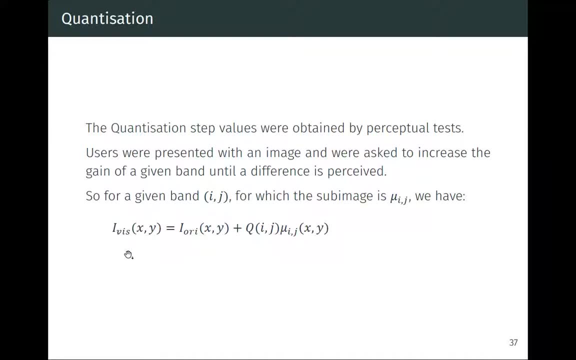 coming back. so, mathematically, this, this is what happens. so you have the. given these two pictures, the original and the degraded one. and the degraded one is obtained by taking the original, multiplying by this quantity, by this factor and multiplying by the sub band itself. we're looking at and we record, when you know, with 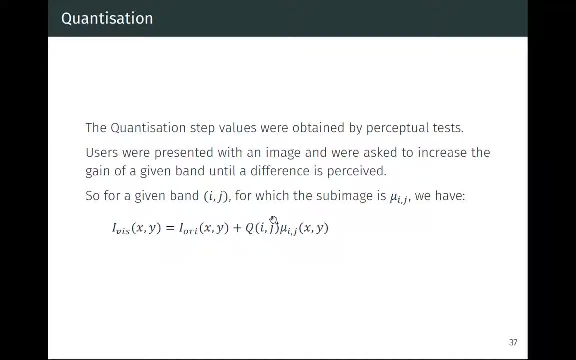 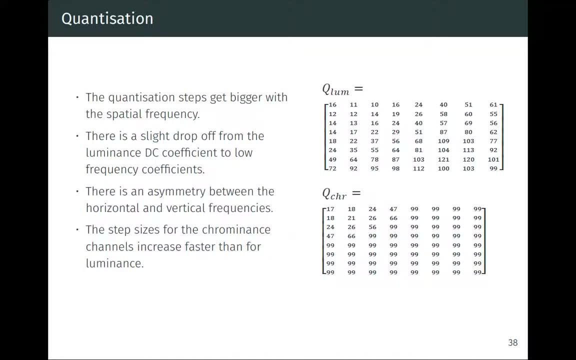 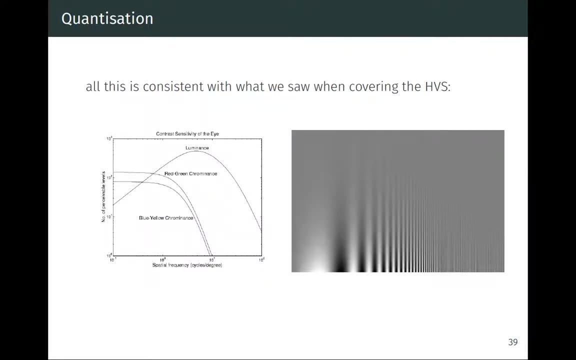 threshold for which people start to notice a distraction, and that threshold is exactly the quantization step we're looking for. all right, so it's quite a simple experiment. so they've done that for a lot of peoples and for a lot of different, to all sub bands, and this is what you got, okay. 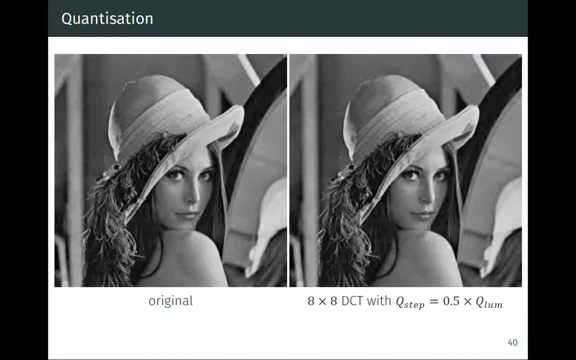 all right. so just to show you a few differences here. so on the left the original, on the right the 8 by 8 DCT, with quantization following this kind of a dynamic quantization step. okay, so Culeum in this one where you apply. 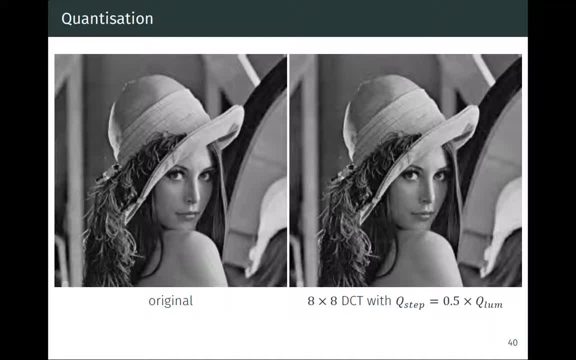 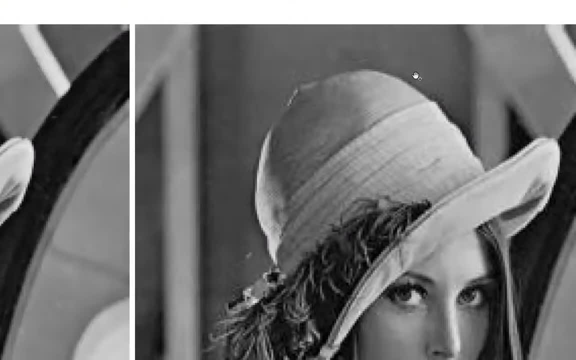 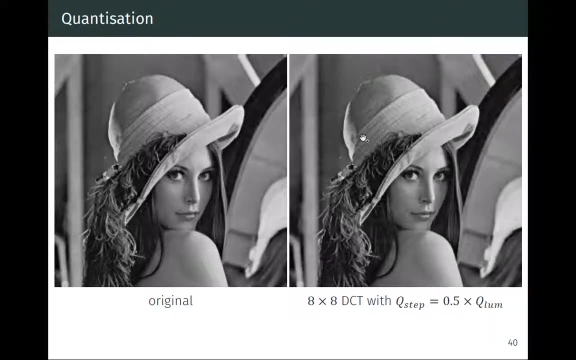 different process or the different Q step for each of the sub bands. okay, so you don't apply the same Q step everywhere. you'll be a bit more discerning. so yeah, it's not. I mean, it's kind of hard to see the differences between all those. so this is with Culeum and this is this quantized step at the distance. you 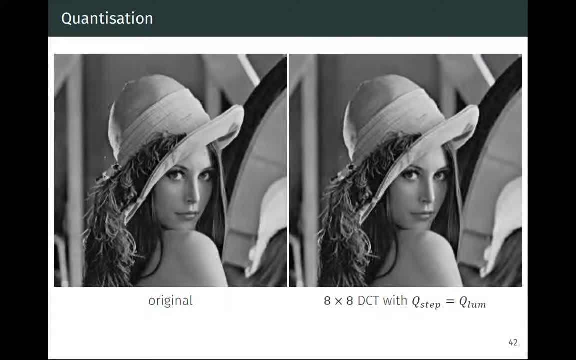 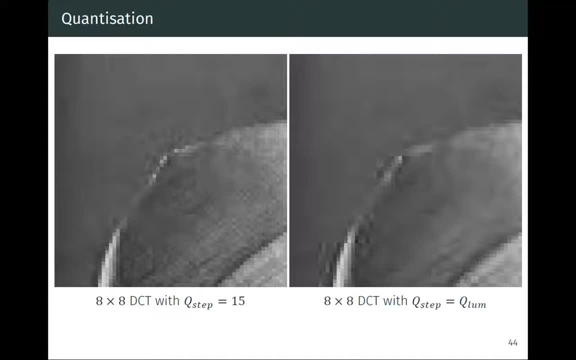 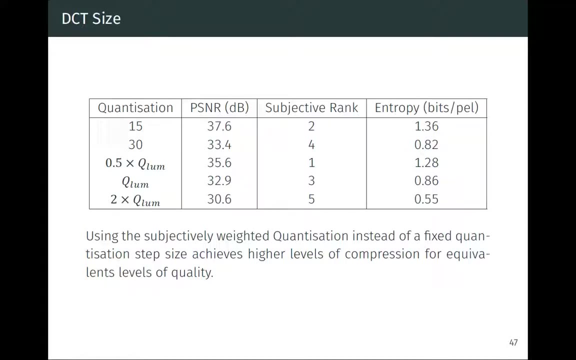 are people. we don't see a difference. you would have to look in more detail in the slides. but yeah, this is you, this yeah, whatever. so obviously, when you do compression, like you, there is a lot of these problems of how you know the objective metric gives you, which is one. 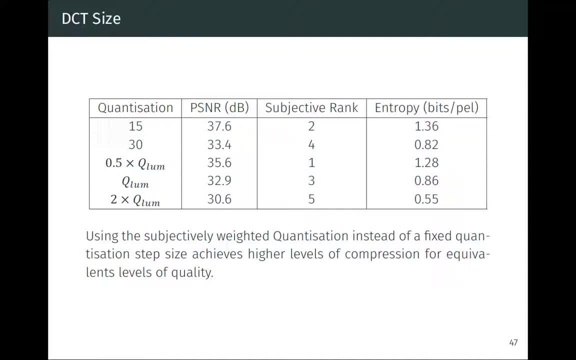 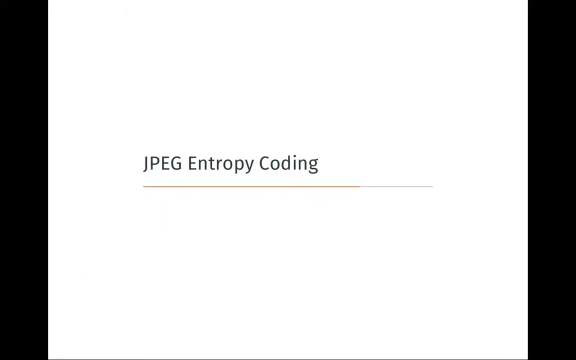 thing and how you have subjective ranking, in which case you need people and you know, you know pile of people ranking the different versions, and then you decide, okay, all right, so that's kind of it. for one example, today, for 99% of what jpeg is, okay, that's kind of what you do, so you 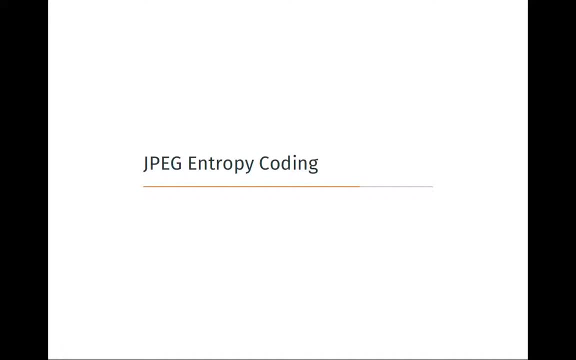 take your pictures for Hunteree color palette, for example, the quantization of Google dell. so here you learn a bit about the 4.0. so you take, split your pictures into blocks, use a DCT transform. you have all this exerted versions of doing that new quantization. you do quantization differently on each sub bucket. 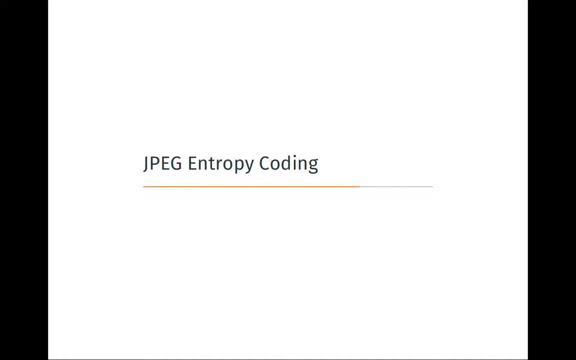 based on quantization step: learn from human visual system and and then you have quantization. unfortunately, some of them have a little bit of a good feeling about. So the last step, once we've done that is, you still need to do the entropy coding. 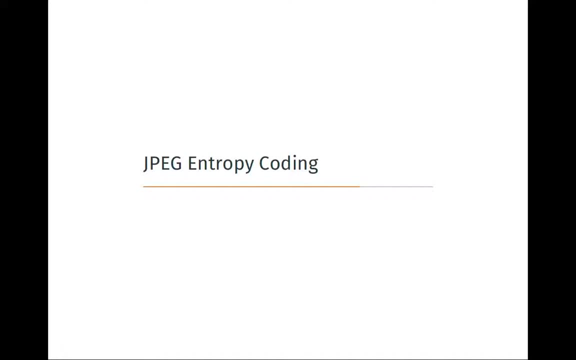 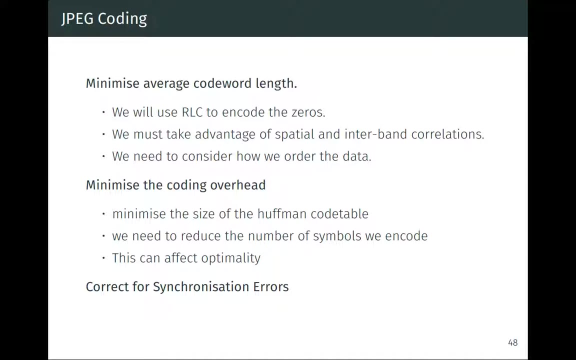 So remember, that's the last step. you transform your picture, you quantized it and now you need to take care of the entropy coding, And now you have a number of considerations to have. The first thing is: well, the main problem is: how are you going to deal with the bands? 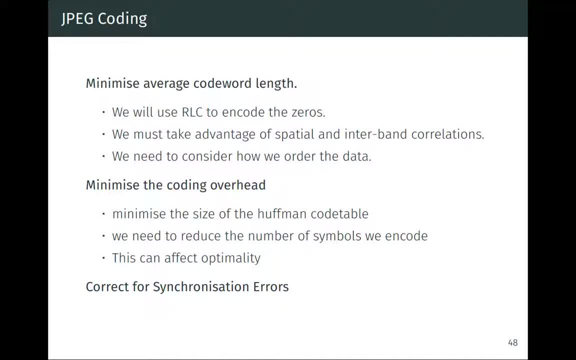 Okay, so far we looked at. you know you have 8x8 DCT, so you have 64 bands and now you replace blocks by 64 numbers and each of these numbers have obviously a different meaning. So when you use Huffman or any of the things you want to use, 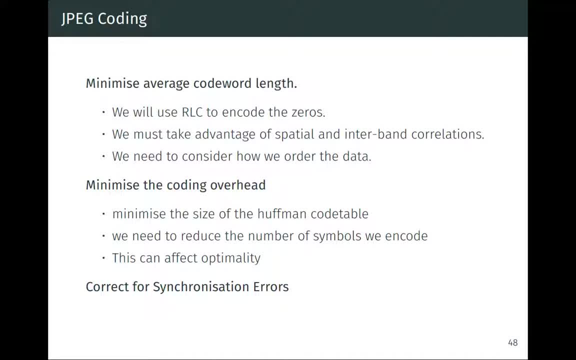 then you probably want to do things. you need to take that into account, okay. So you know, a naive way would be to say: well, I looked at the 64 sub-images, I get. okay, So per band sub-band I get. you know, we compute an image. 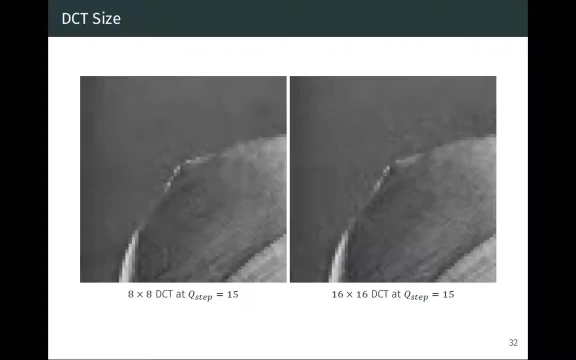 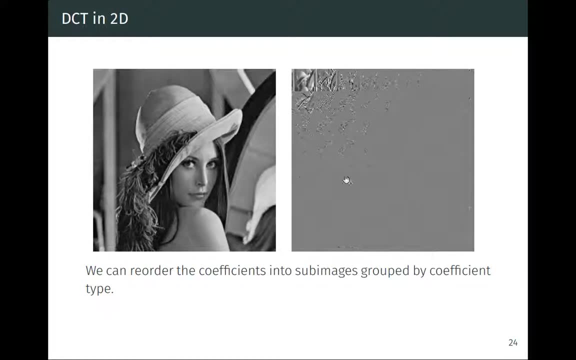 and so you know that would be coming back to that, you know. So, looking back here, if you look at the 8x8 DCT, you can recreate all these 64 images and you could think: well, maybe I should compress. 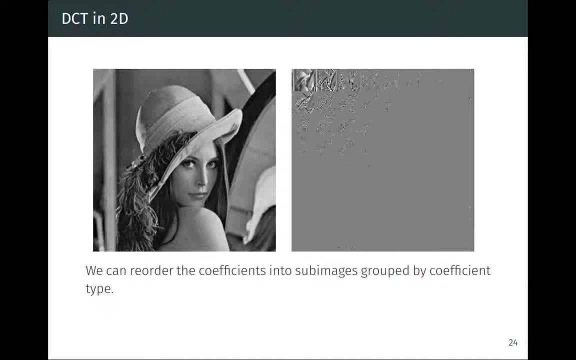 it, you know, and then you can do the same thing. So if you compress each picture, each of the 64 pictures, independently in its own Huffman code, yes, So, DCT, you don't lose any information. okay, as long as you work. 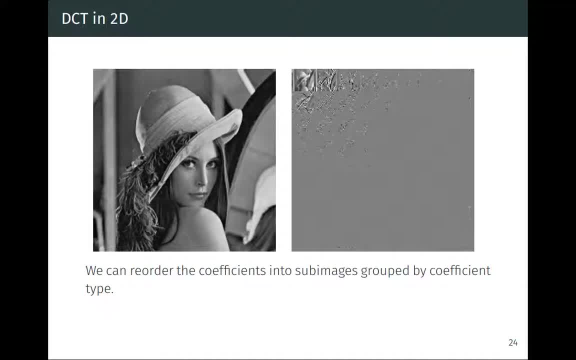 you know floating points, accuracy and so on. okay, So, as usual, the transform there you can come back. you know the inverse: DCT will bring you back to where you are, It's just the quantization is really the one. that destroys the information. So you know you can come back. you know the inverse DCT will bring you back to where you are. It's just the quantization is really the one that destroys the information. So you know you can come back. you know the inverse DCT will bring you back to where you are. It's just the quantization is really the one that destroys the information. 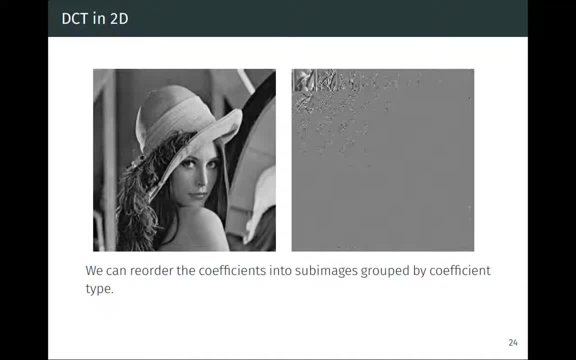 That brings you to lossy compression. So all right, so at this point you've compressed, you've transformed your picture. this is a transformed version. and you say: quantize them. and you want to apply Huffman. and you know what do you do. I mean, you could apply Huffman or whatever zip algorithm. 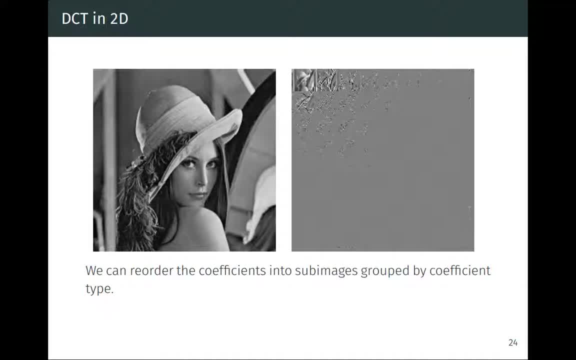 on the entire picture on the racks and just say this is what you have. Or you could try to say: well, each of the 64 images has its own behavior, so maybe I should learn from Huffman. I haven't applied different Huffman code. 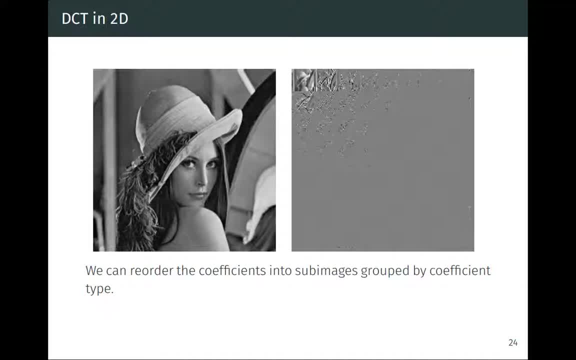 for each of these 64 images. Okay, so effectively, instead of one Huffman or one zip, you apply 64 different zips, zip compression on the 64 subbands And you can see: okay, there's definitely something that can be optimized here. like you need to take a decision on how you do it. 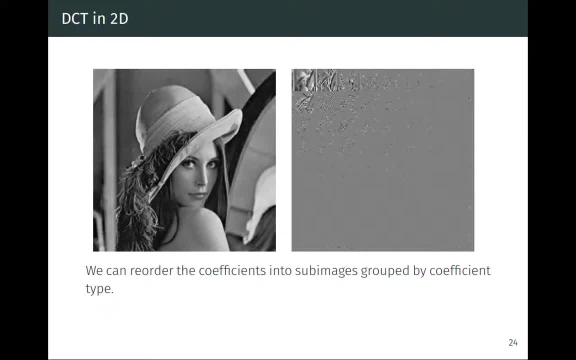 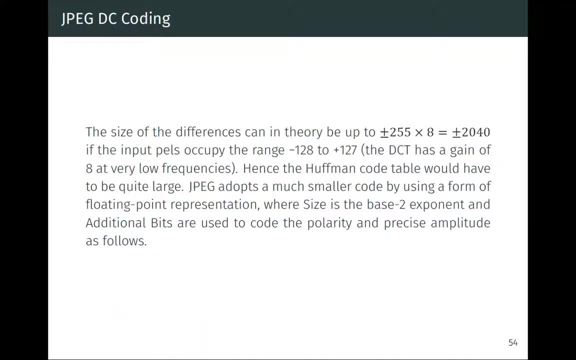 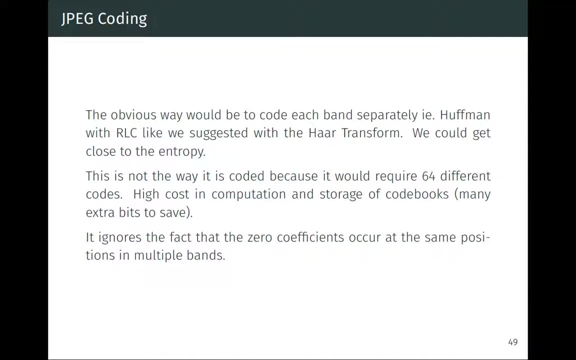 but you know there's it's not trivial to think how you go about that Um. so the way they approach it in the, so coming back um, in, in, in, um, in, um, in JPEG is um, sorry to apply this kind of zigzag pattern okay. 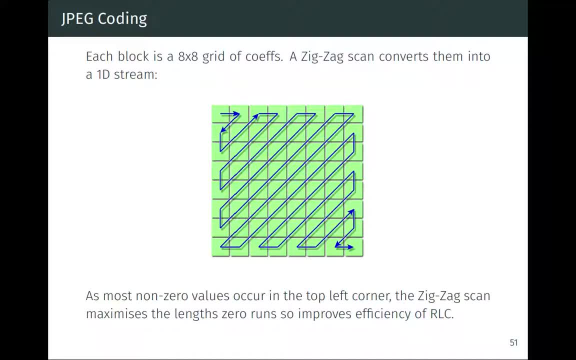 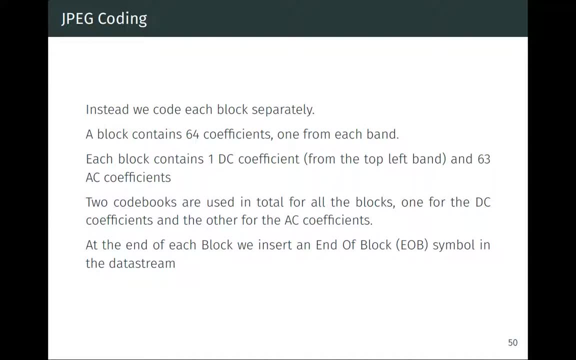 um, all right, so there's. there'll be a lot of things going on, so the sorry. coming back here, the first thing they're going to do is to look at, to analyze the image. okay, the DC coefficients usually behave differently from the AC coefficients, So that 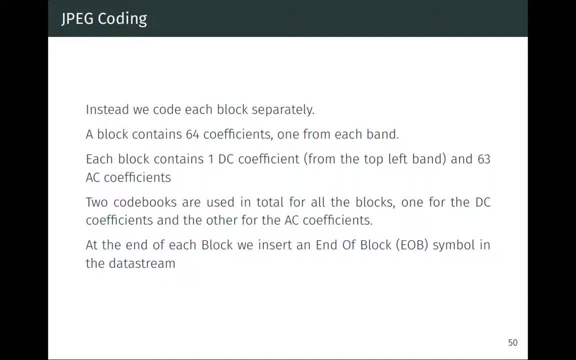 makes sense. remember, when you look at the pictures on the DC coefficient, we saw like the DC coefficient was very strong, okay, like that's basically your low, low, your low pass image, okay, and all the other ones are kind of you know, remember the Haar transform, if you look. 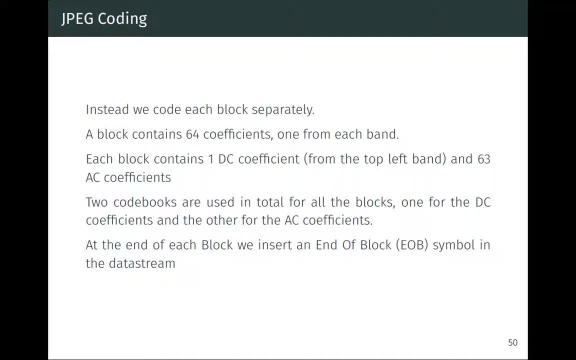 at the low, low pass. that's kind of a subversive you know resized version of your picture. and the other bands are kind of very much different in nature. okay, they're all kind of almost zero with you know, only at the edges. So it kind of makes sense to have two different. 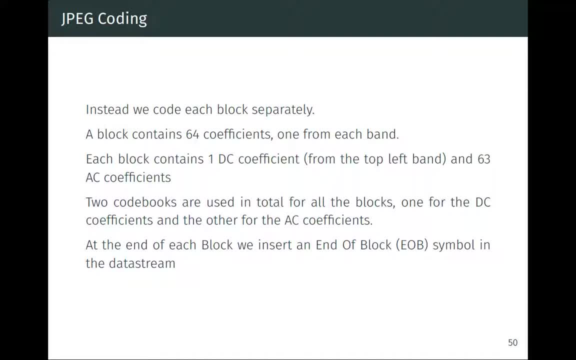 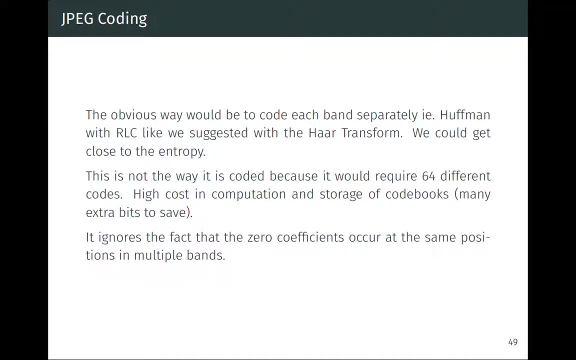 strategies. one of these, which is for the, uh, the DC coefficient, so the low, low pass, and, uh, you know, a separate strategy for the all the AC coefficients. okay, so that's the first thing. um, the, um, the. 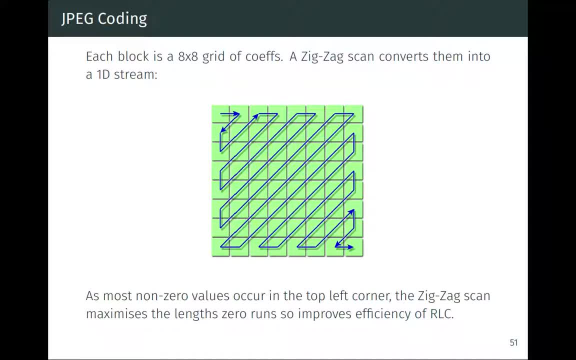 all right. so when you look at the AC coefficients, so all the ones that Haar kind of higher frequency than zero, you get something like that. okay, so you have your um, all your coefficients organized in your eight by eight grid and going from the, you know, the DC coefficient. 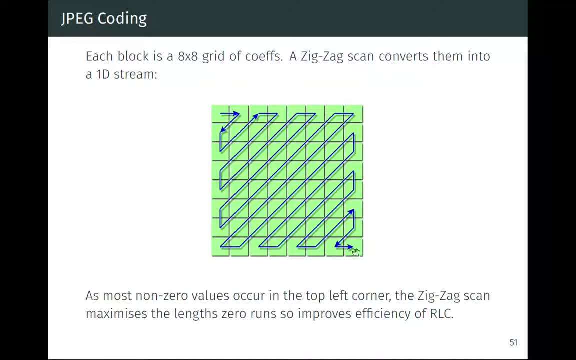 here. if you want to be um to the highest um frequency here and the way we transform the picture, okay, so we will do a code, that is by using this zigzag pattern. okay, so we are going to um. so you have your 2D block and you need to transform that into one of these stream. 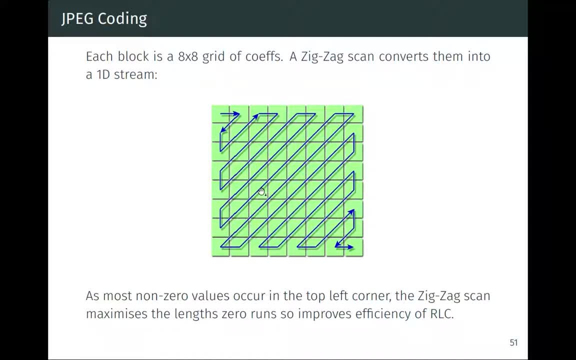 and we're going to rearrange all the coefficients along this zigzag pattern. so we're going to start from the lowest frequencies and zigzag along similar levels of frequencies, but going back and forth between the x and the y frequencies. okay, and you finish by the. 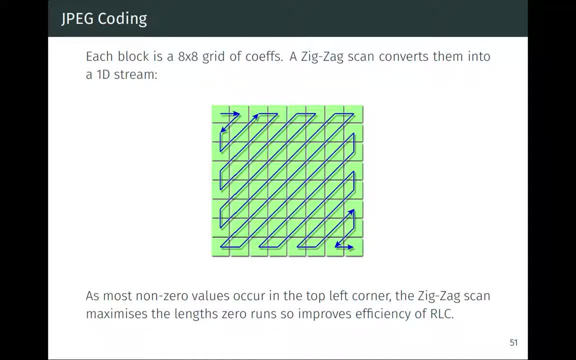 high frequencies both in x and y. does it make sense? all right, so I'm just going to realign all the um, all the, all the coefficients. okay, so here's the matrix of all my coefficients and I'm 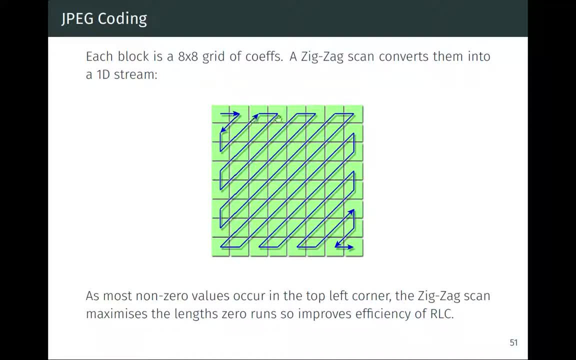 instead of going from you know, reading it, uh, row by row, I'm going to read it in this particular zigzag pattern, and the reason why you want to do that is because what we know from, uh, from what we've seen before, is that all the most blocks, all the energy, all the non-zero um. 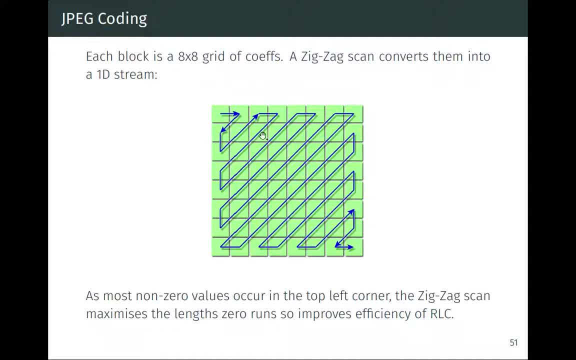 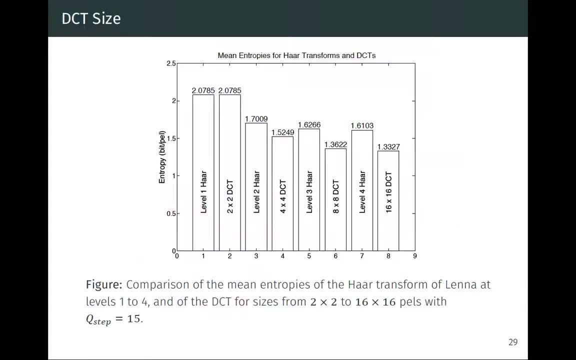 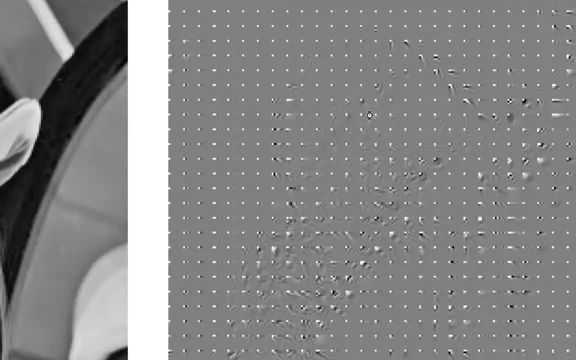 coefficients are in the top left corner, okay. so all the values that are um high, okay. I just want to show that again when you look at the particular block here, all right, even in the ones where there's a lot of things going on. 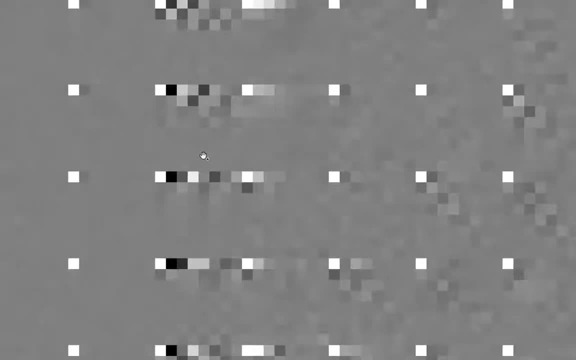 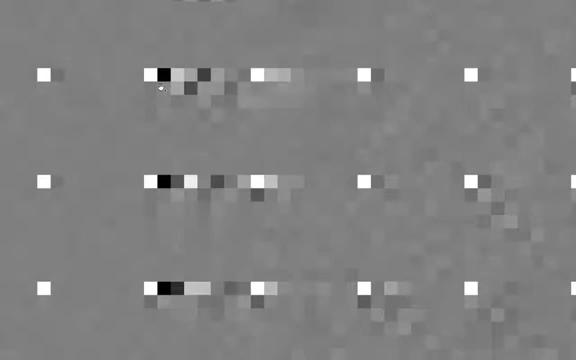 you can see if you extract just that particular block. so you see, the dc coefficient is very specific, okay, but all the other ones kind of only happens in this um top left corner, okay. and you see, here when you're at the bottom, you really have nothing. it's mainly zeros. okay, so you have a lot of zeros. 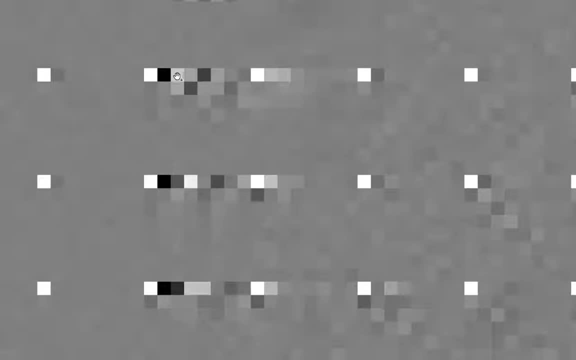 towards the end and by reorganizing into the zigzag pattern. what happens is that after rounding- most likely- uh, towards the end- you're going to have a lot of zeros. okay, so, in your sequence, you're going to reorganize all your coefficients and you're going to have a lot, lots of non-zero. 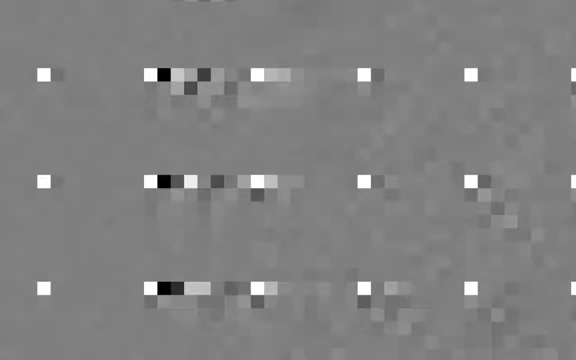 coefficients at the beginning of your, of your, of your zigzag pattern, and at the end of it, when you read it, you're going to have loads of zeros at the end. all right, make sense. So you start from the top left here, and you have lots of non-zero values and then, as you go down, 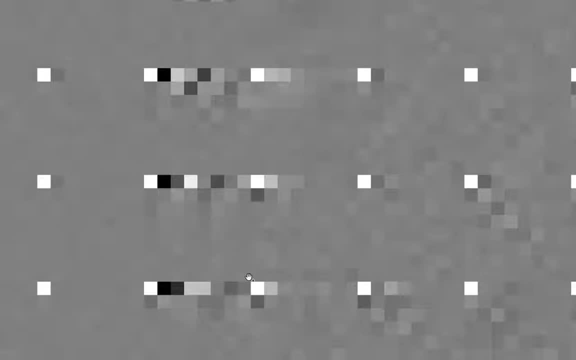 after here, for instance: okay, after quantization, all these guys will be zero. okay, so somehow you reorganize your data in a way where you kind of split and say, okay, at the beginning of my stream I have lots of non-zeros and at the end I have probably lots of zeros. 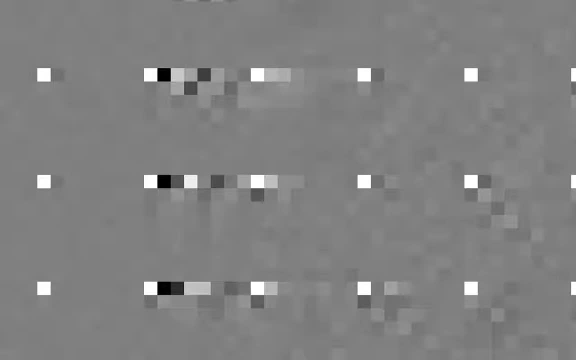 and by doing that, then I can use run-length coding. so we run run-length coding. I just start to say: um, you know, here's a bunch of- uh, non-zero values, But here I have eight zeros in a row that will come after you. okay, so you have one code that. 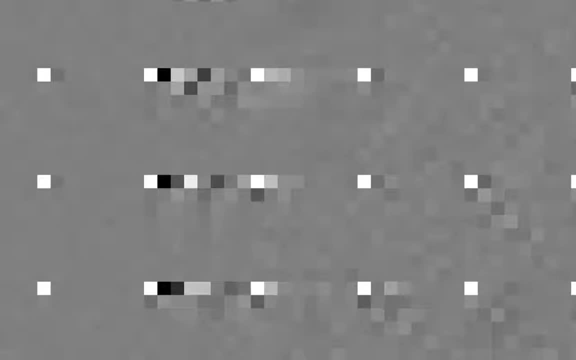 tells you you have eight zeros ahead of you, you have 16 zeros, and so on. okay, So this zigzag pattern is quite an important trick from JPEG. allows you to reorganize your coefficient in a way that increases the number of zeros you have in a sequence. and because you've done that, then you 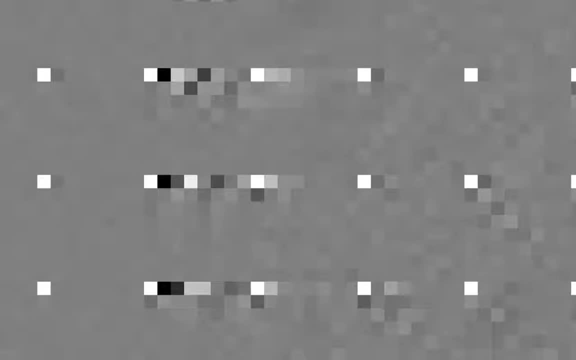 can use run-length coding very efficiently and you know, if you look at this block, for instance, maybe two other ones that are, you know three of the ones that are non-zero, but then after everything is zero, okay, so the way you code that block would be: you know, code this guy, this guy. 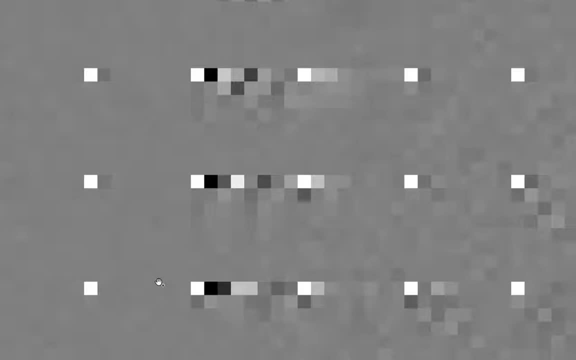 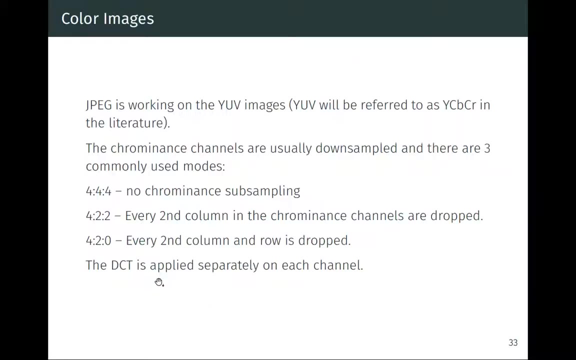 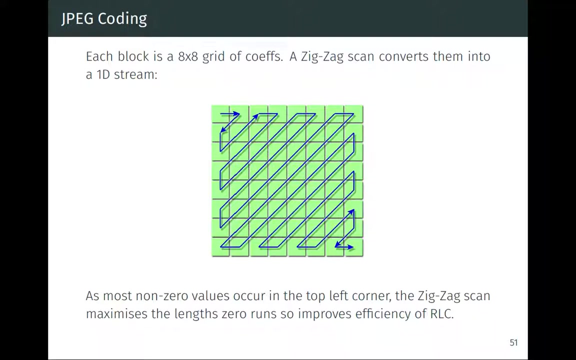 this guy value and then you say you have 16 values of zero afterwards. okay, so it's a very efficient way of coding it, Right? so this is the first thing, okay. The second thing is: how are you going to encode the so, right? so the AC coefficients will be mainly encoded by. 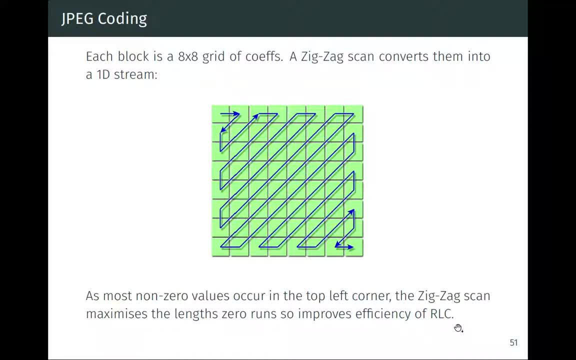 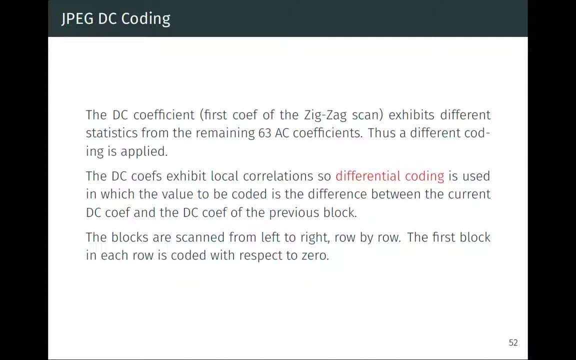 thanks to the run-length coding. okay, so it says here: run-length coding The DC coefficients. okay, we know that there are. you won't have that many zeros. okay, so you have values all over the place, because basically it's just a. 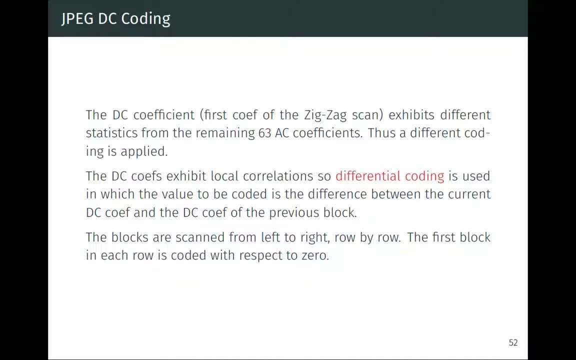 sub-sampled version of your original picture. So what we do then is kind of almost like a in Haar. you know, you have a multi-level transform where you look at that low pass that you know sub-banned and encode it again. we do some kind of sub-version of that in the sense. 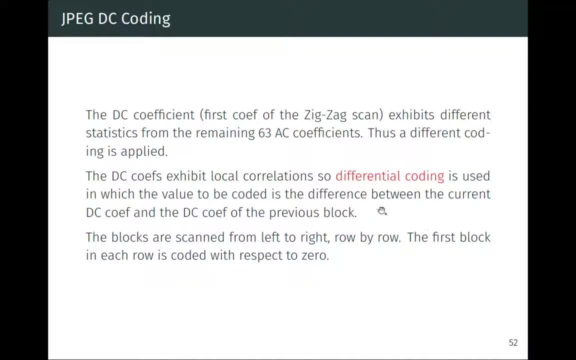 that we look at the DC coefficients and we're going to apply differential coding on the DC coefficients only. So what that means here is that you're going to look at in align, okay, so you. So you process a row of blocks, okay. 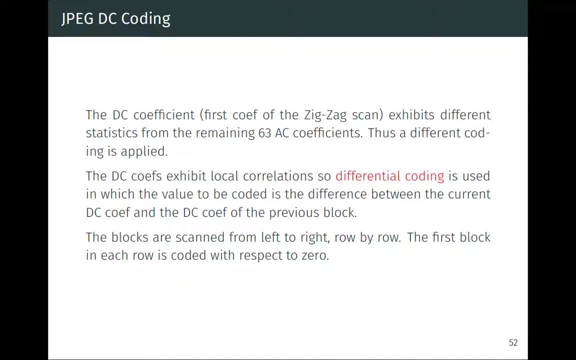 So you have, I don't know, 20 blocks along the x-axis And you look at the DC coefficient for each of these blocks. Now you have 20 values, 20 values of DC coefficient. So if you apply differential coding, 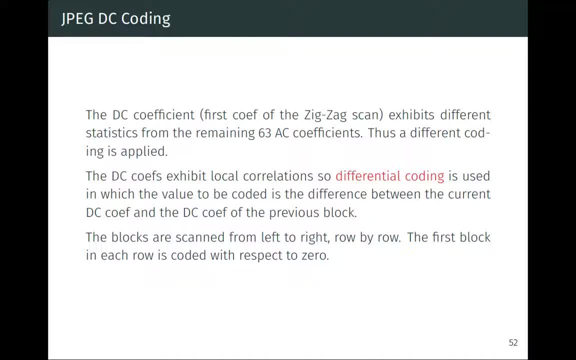 so we just do the difference between the blocks. then you can get a good prediction of what the next DC coefficient should be. all right, And so this is what you do. okay, So you apply differential coding on the DC coefficients. So there you go. 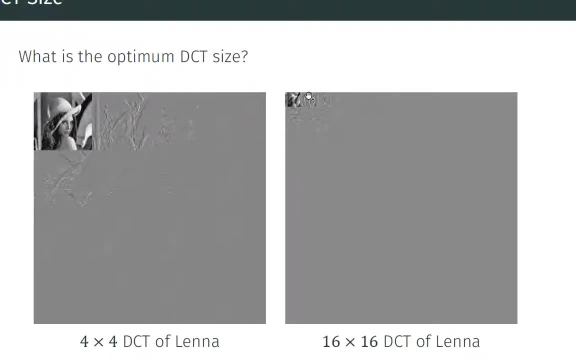 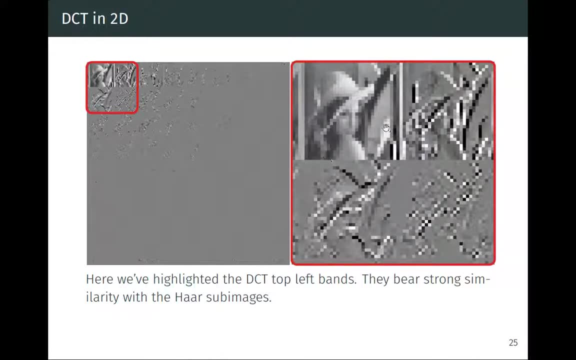 When you look at the. So I'm looking at this picture here. okay, The question is: how do you encode that picture? How do you be smart about that picture? And what I'm saying here is: we apply differential coding on the DC coefficients. 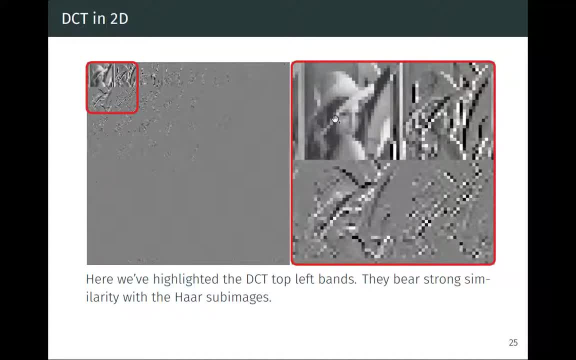 We apply differential coding on that picture. Remember, differential coding is kind of the first version we've seen before the heart transform. okay, We take the pixel on the left minus the pixel on the right, or vice versa, and you just encode that difference. okay, 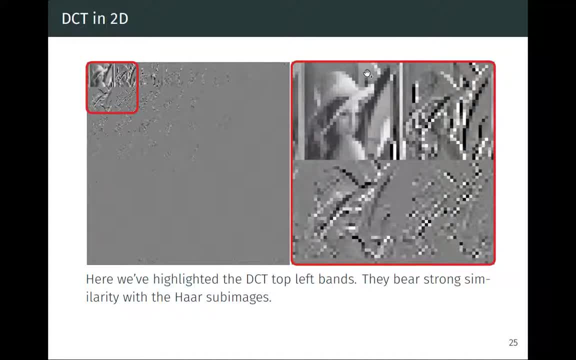 So for the DC coefficient, there is this special scheme that you apply on this picture. all right, Does it make sense? So I'll say that again. all right, The AC coefficients you apply. you have this zigzag pattern. you apply on a block level basis. okay, 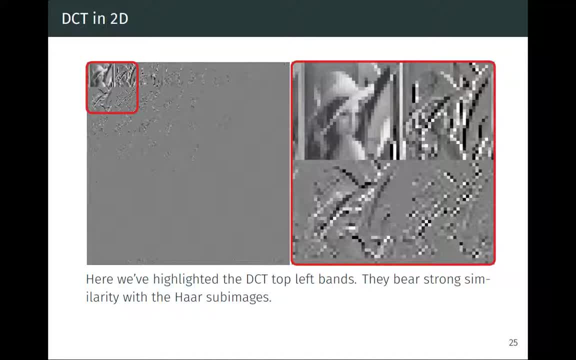 So on AC coefficients, so all these higher frequencies, we just look at- you know this zigzag- and just apply that on every single block independently. To compute the DC coefficient of each block, we are going to depend on the other blocks, okay. 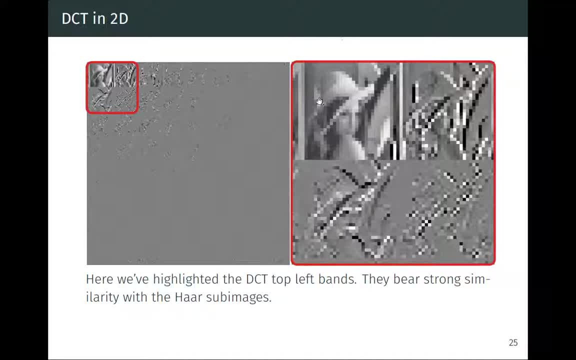 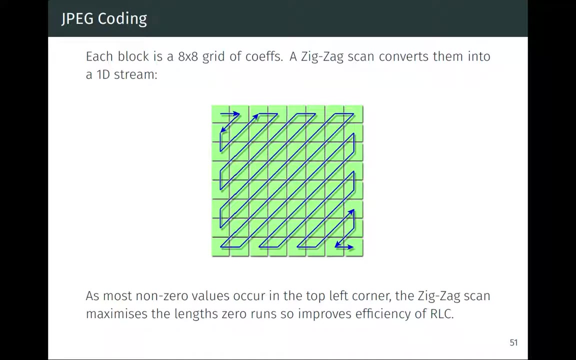 So, in fact, what we're doing is we're building this picture, this sub-band image, and we're going to encode that using differential coding. all right, So that's how we do it, Okay, so this is the main tricks. 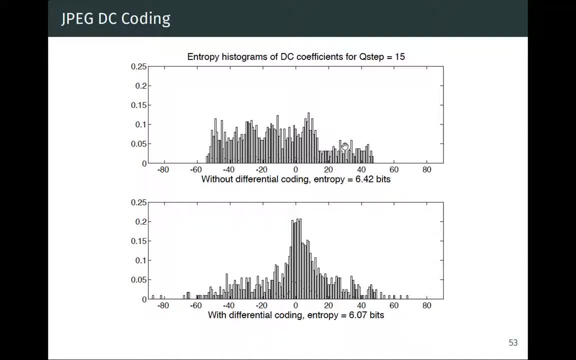 So kind of coming to the same kind of grasp we had before for differential coding, okay, So this here's the histogram of the DC coefficients on a picture for Q-step of 15.. And so the same histogram that you have for the original picture, okay. 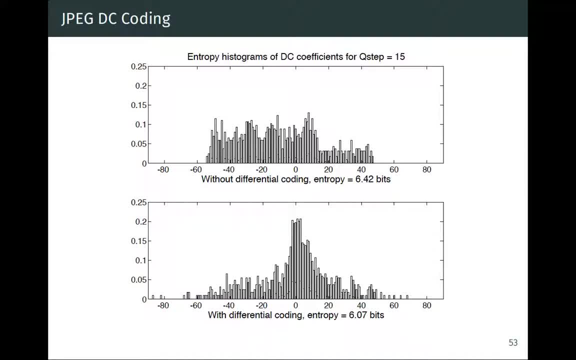 It's called the same. okay, That's the histogram of your low-low band, okay, And what you have here is the histogram of the difference along the x-axis between the pixel on the right and the pixel on the left, And, as you can see, you have the same kind of characteristic. 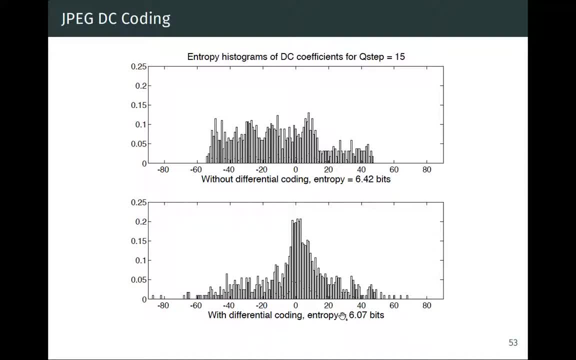 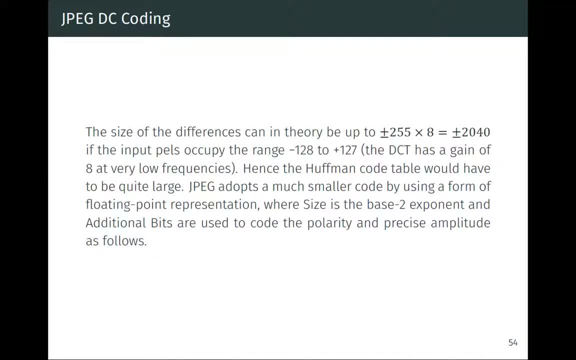 where most of the values would be around zero. okay, You have this tail-off effect. So that's the number Right. so that's the two main mechanisms applied. okay, So the zigzag pattern and the differential coding. The last bit is on Huffman. okay, 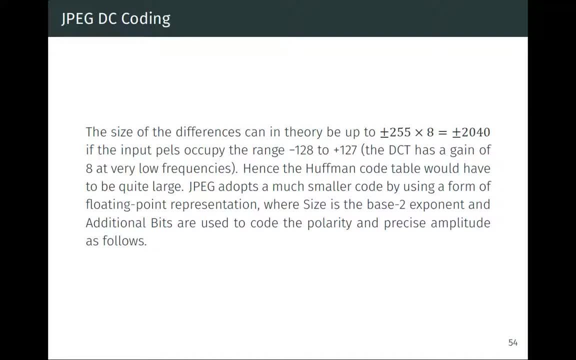 So in theory you could use Huffman. The problem you have is you generate lot more symbols that you had before. okay, So when you look at the um, the, the, for instance, I think that's for dc coding. for dc coding, okay, so you apply dct. 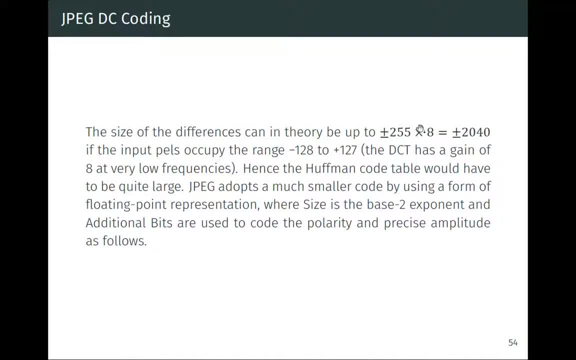 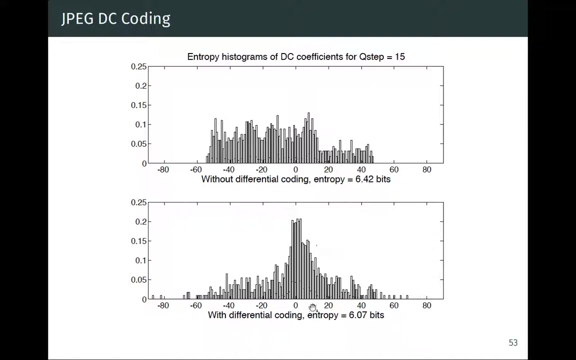 because the dct has a gain factor of eight. you do the average between eight um eight numbers on the dct, one uh 1d. then really the number of symbols you have when doing the difference is um 255 by times plus or minus here. so really have the range of values you have when applied on the dc uh. 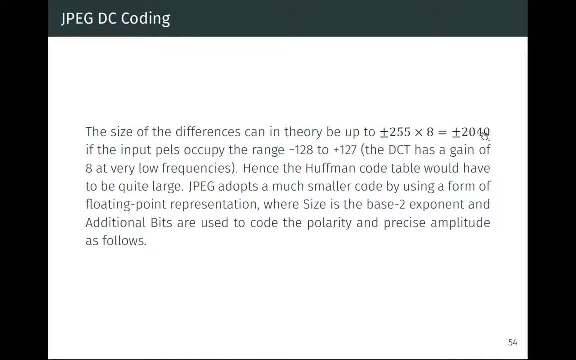 coding is really, you can go all the way from plus 2040 to minus 2040.. I just remind you of that. in the hat transform, you know, for instance, like when you you extended the range of symbols you had, you set it from 0 to 255, and when you apply the hat transform, 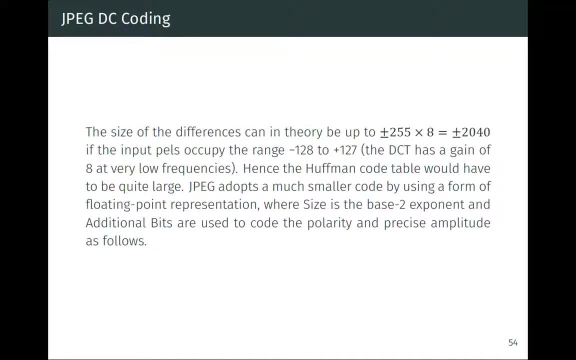 I think you went from 0 to 502, or minus 512 to plus 512. okay, so when you apply the transform, what happens? that you can actually increase the number of symbols you can have. okay, and even after quantization, uh, you might end up with more uh symbols. and the problem here is, like your number of symbols you have, um, just for the 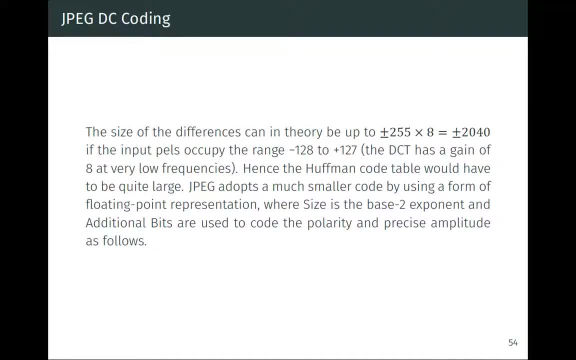 dc band uh is actually quite high because you have basically 4000 different number of symbols. okay, and now you need to um have a huffman code table, uh, given in the header of your file. so when you give a jpeg image, you need to say here's my huffman table for the dc coefficient and right there you need um to. 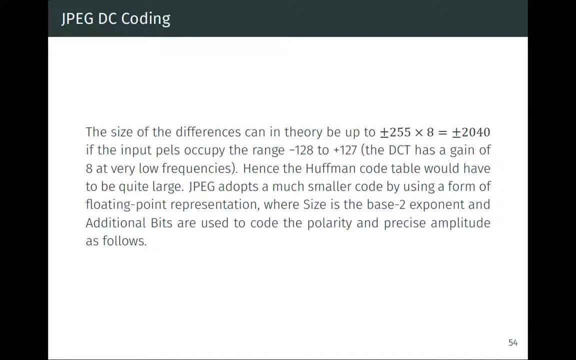 describe what 4000 symbols. you know the table for 4000 symbols. okay, 4000 symbols, it's quite out of symbols. and you know that's already a few kilobytes of your file, taken just in the dictionary itself, which starts to be quite heavy. 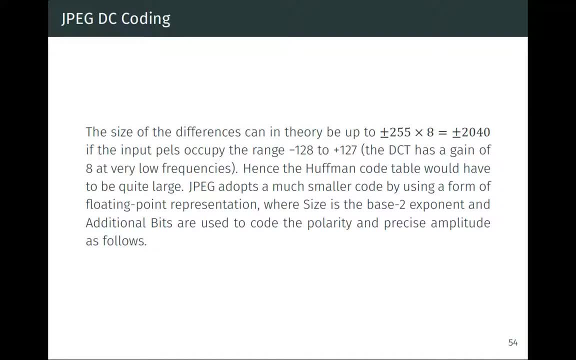 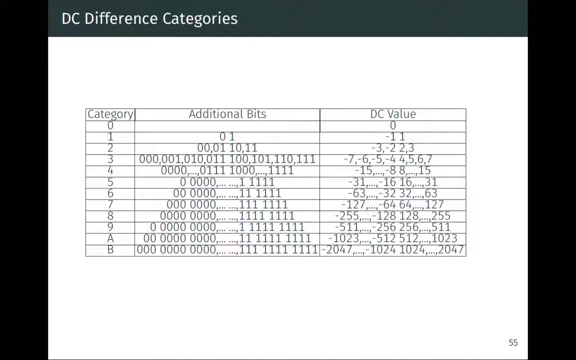 so, um, in the in the community, in the jpeg community, you know, i won't go into much detail here- uh, i invite you to read the slides because it's quite boring, um, but basically they come up with some kind of built-in version. okay, so they, instead of designing the optimal huffman code, 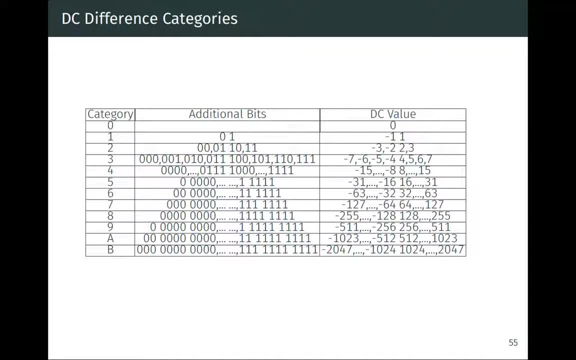 uh, they say: well, here's a, here's a code for you. and uh, here's a recipe of how you get that code okay. so they kind of have a, a formula about basically lookup tables here to say: if you're have, uh, if your coefficient is in that range, then you know, this is, this is how you should code it. 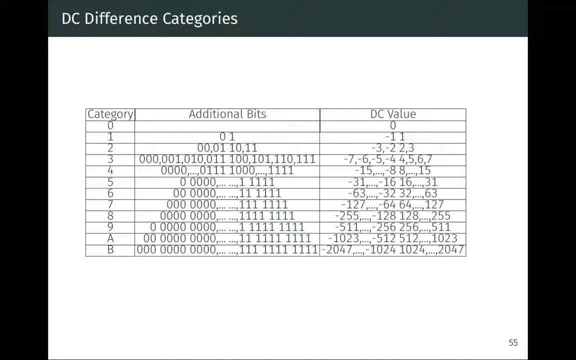 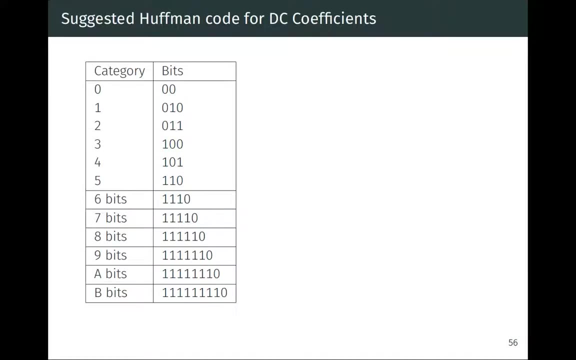 okay, so for each um they have a mapping or a kind of a manual mapping between the value of the coefficient and how you code that into number of bits. all right, say that again. um, so it's this story. this is all the the words down here. um, but basically, okay, this is an example. if 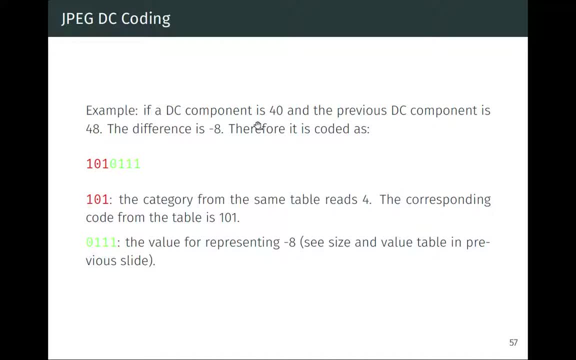 you have a coefficient which is 40, okay, so that's the, the value of it, the after compression, and you know, transform and so on and um, the next one is 48, so you do the difference between them to do the difference coding, so you get a difference of minus eight. okay, so 40 minus 48 and minus eight. 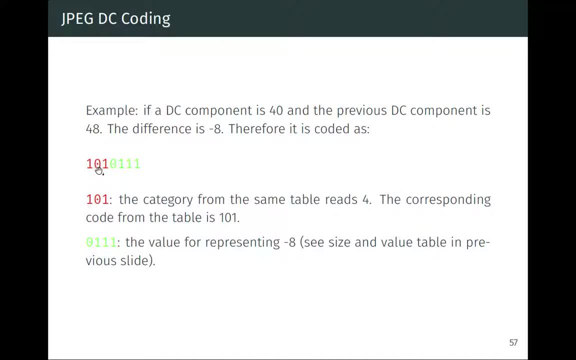 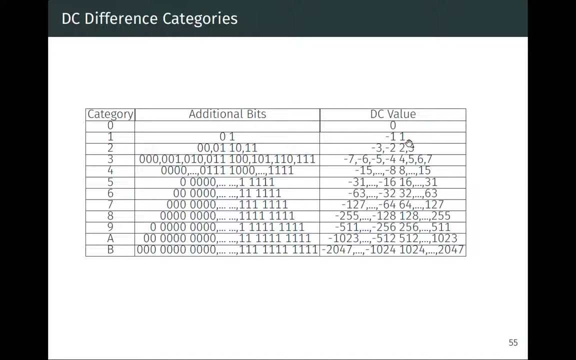 will be coded um as one or one or one one, one, okay. and so basically you have um two parts, okay. the one, part 101, which tells you how big the number is. okay, so, all right, look here at this lookup table and say i have the value minus eight. so you look. 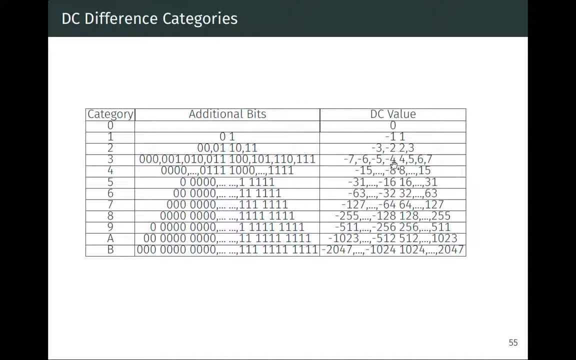 i'm here in that row, okay. so on, look at the right, the column right. so my value is minus eight. so i know that, um, i'm in category four and range of possible, you know, have all the bits going from zero, zero, zero, zero to one one, one one okay. 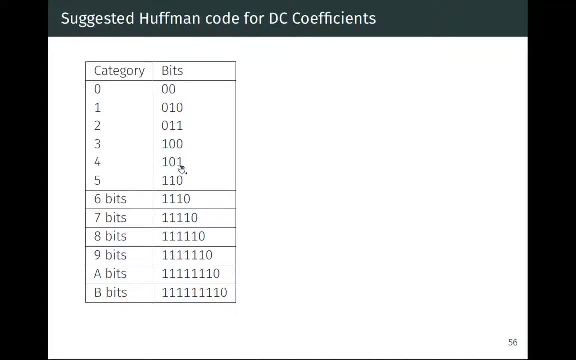 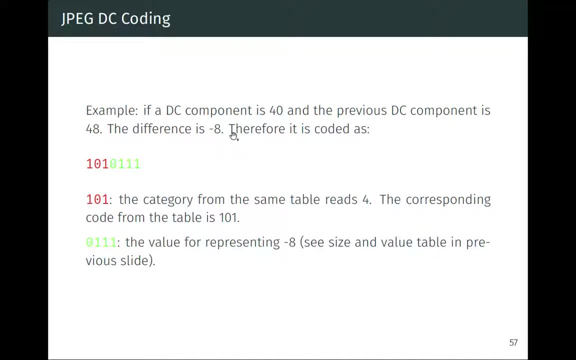 and then in the category four, you read and you say, right, this is this code. so basically what it means? okay, it means when you do the dc coding, uh, you get a number minus eight and you want to. the very last stage now is to transform that minus eight which comes after all. this transform into: 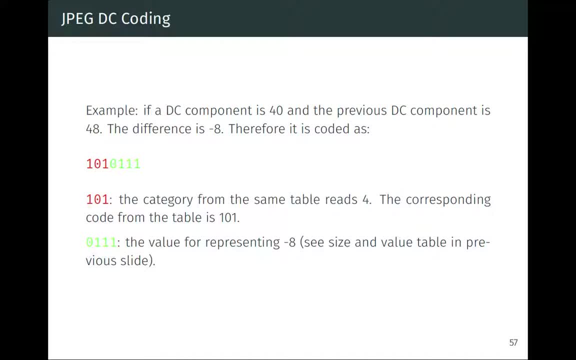 uh binary code. and instead of using halfman, we have now this lookup table, or this mechanism in which we're just going to replace minus eight by a particular code, and that code is: is worked out as follows: with these two, two parts, one looks like the magnitude of the code. 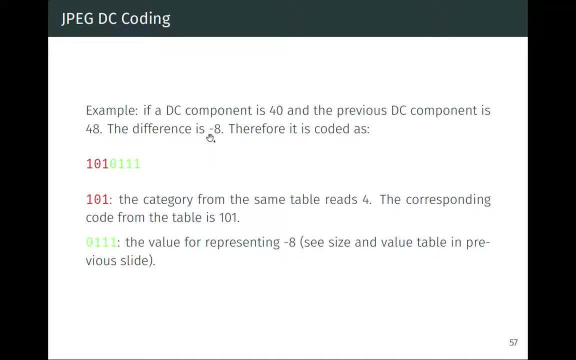 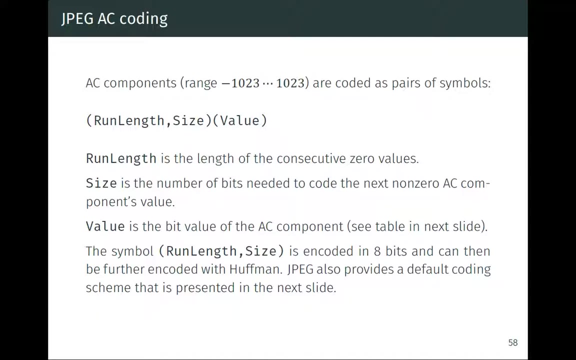 the number. so the bigger the number um, the more the more bits you will need. and the other part gives you the index within that that range. okay, so for the ac coding you have a different scheme, but as well it's a manual process. okay, so you, you have these running coding schemes and um, i won't get into too detailed because it's. 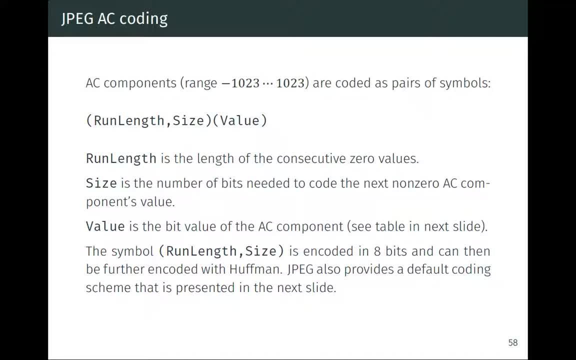 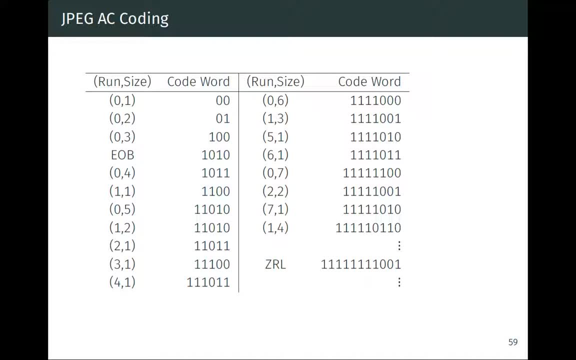 kind of. it's really boring, but it's in the slides and you have to read the slides for that to ask me questions if you have issues. but basically the same story. you have a whole process that tells you how you transform a particular value you have in the ac coefficient. 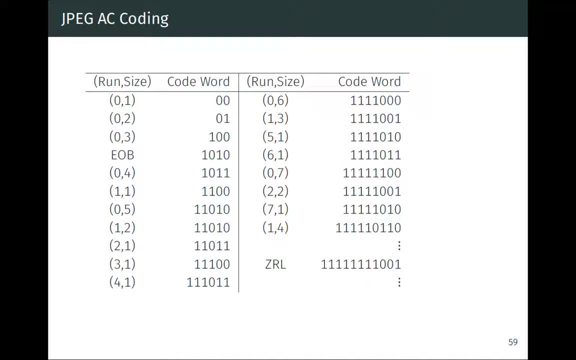 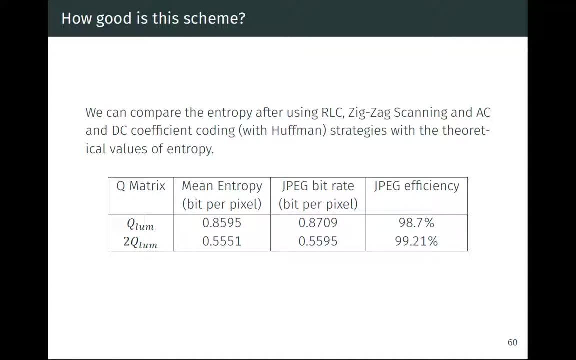 and that you found, and how it relates to a particular sequences of bits. all right, so, um. so how does it compare to? so we have all these hacks now in jpeg implemented, and? um, so when you look at the table here, we can see how the entropy after. 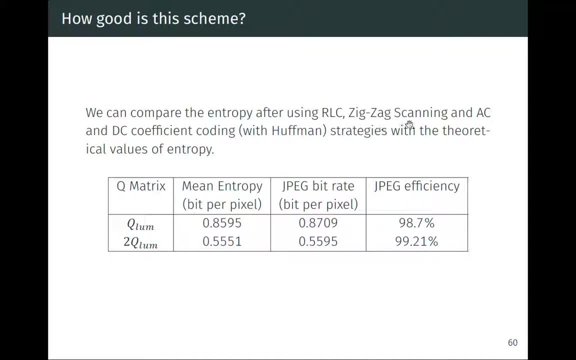 um all our systems, so brunette scanning, zigzag scanning and so on and so forth, with the theoretical value of the entropy. so if you apply the q loom composition scheme on our picture, we find that the mean entropy, so bit by pixel, is 0.85 and what you get with jpeg is 0.87. 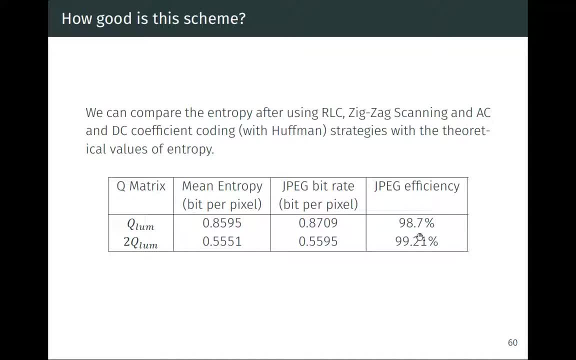 okay. so we have roughly 87 percent of the jpeg value in jpeg. so we have roughly 87 percent of the jpeg value in jpeg. so we have roughly 87 percent of the jpeg value in jpeg. so we have roughly 87 percent- 89 percent accuracy efficiency. okay. so with all this kind of manual tweaking and all these, 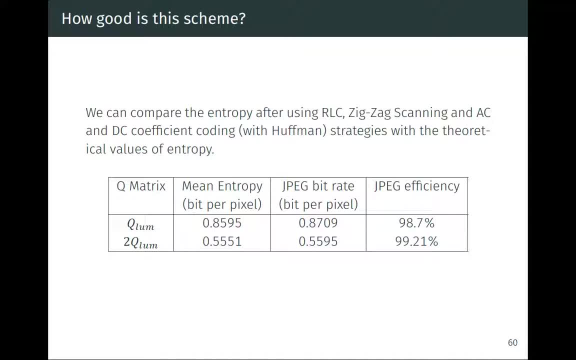 rules done by hand, we still get very close to what the optimal rate is for, uh, for that, okay. so it turns out all this, you know, zigzag and scanning and roc and so on. uh, it's quite efficient. okay. so you know, for any given picture, you reach something like: 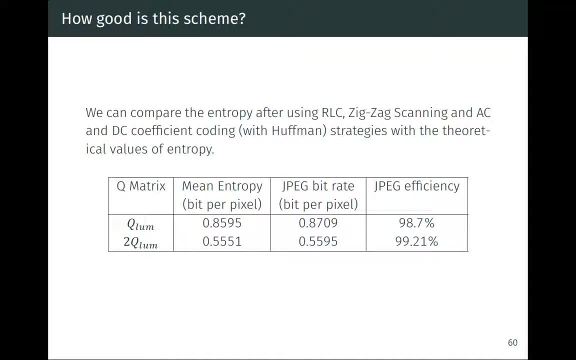 99 efficiency. so you won't get that much by using half man. okay, that's the whole point here. if you use half man, you get one person, maybe the last one percent or closer to one last person. but then you have to encode, put all the header files, all the tables in the header files, and that will take a. 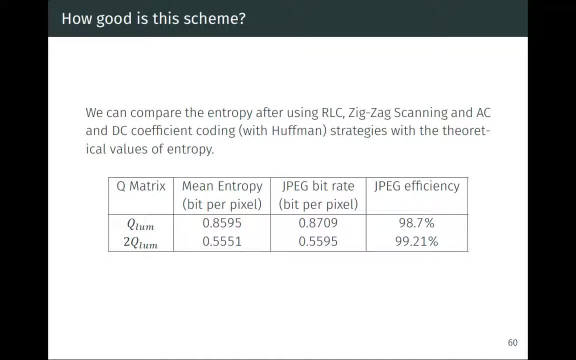 lot of your space. okay, so by using formulas that you know, by all agreeing on the same coding schemes, you save that header. you don't have to put that header, you don't have to add that information. all right, um, that bit, okay, thanks.